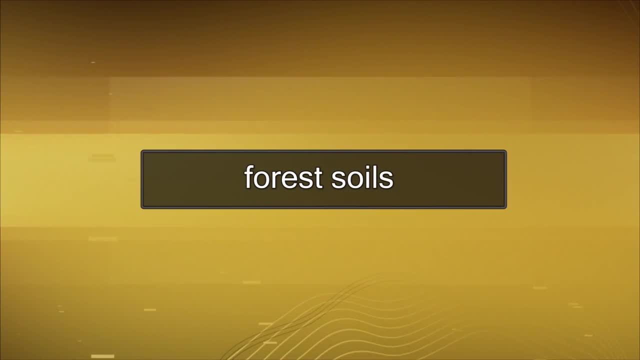 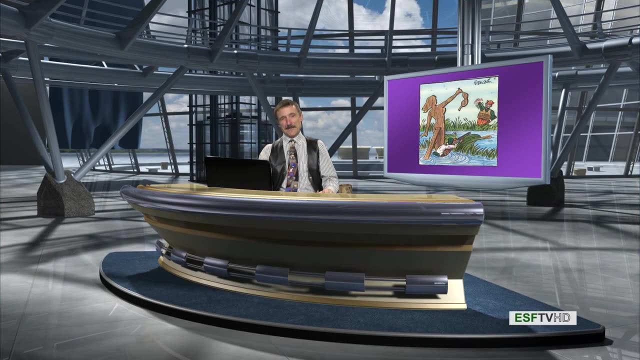 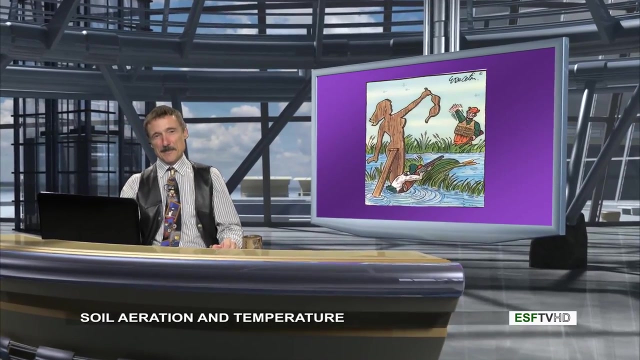 Good morning FOR 345.. It's time for soil aeration and temperature. I'm here in the cloud city of Bespin just before the Jedi Council meets, and before they meet, I thought I'd get this lecture in. So this is getting near hunting season, and so I have one of 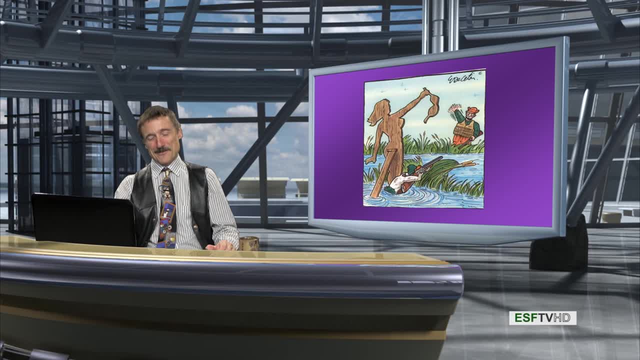 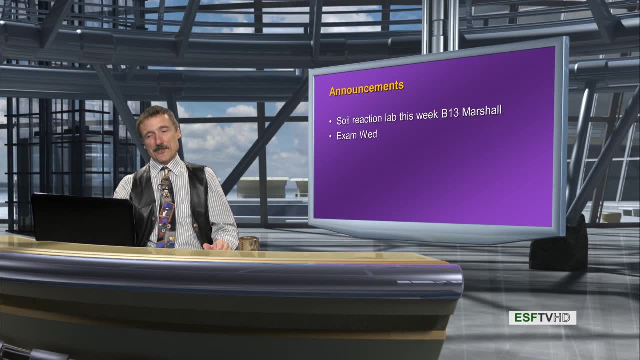 my favorite hunting comics, as you might see, and so when the duck hunter is hunted or when the, this is what happens. Well, this week we are doing soil reaction, and so we're back in B13 Marshall after our cation exchange. and remember, the exam is Wednesday, If you. 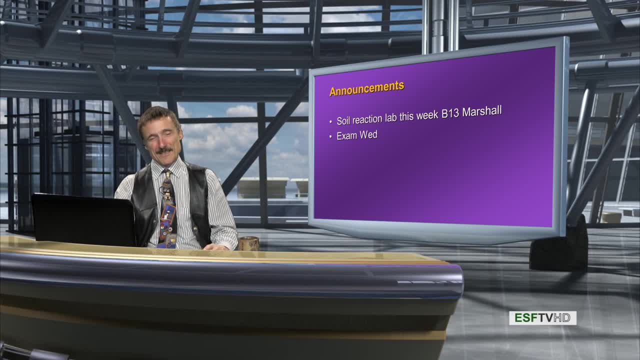 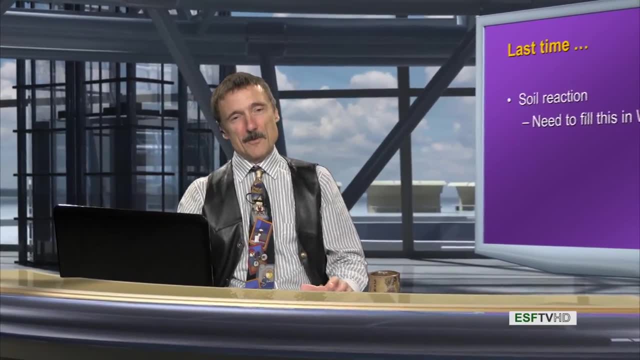 aren't remembering that, then you're in trouble. So the exam will be Wednesday morning. Show up on time, even a little bit early, get to your seat and we will get the exam to you. So what did we do last time? Last time we were finishing up soil reaction, Actually. 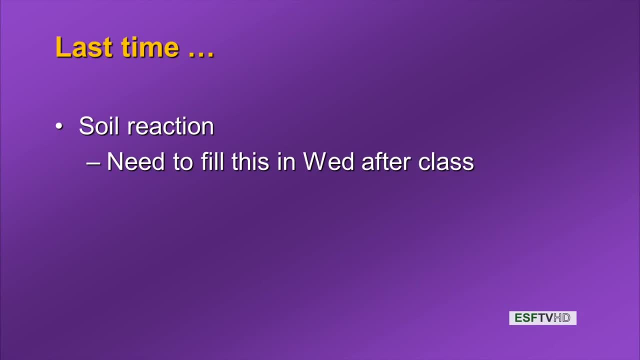 we're kind of in the middle of soil reaction and we'll need to fill this in Wednesday after class to finish up, but I wanted to start aeration and temperature now and let you get through the soil reaction lab. All the stuff that we did last week should enable. 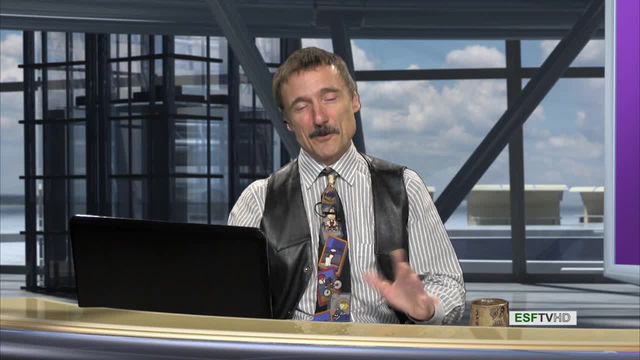 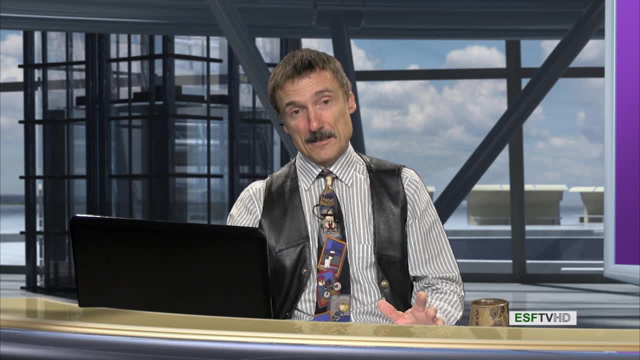 you to get through that lab fairly easily. Well, I wouldn't say fairly easily, but if you have prepared and gone through your notes and you've gone through the web links, this will make a lot of sense. We'll tie that up next Monday in the lecture and then we'll 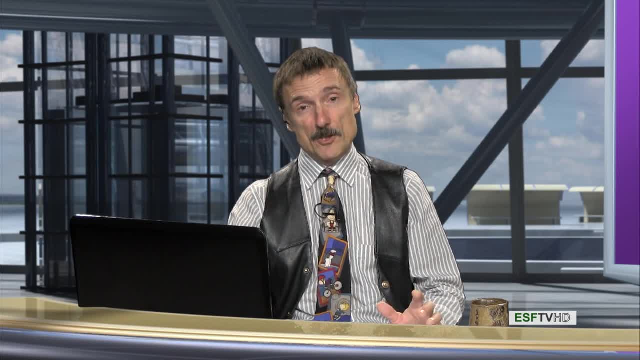 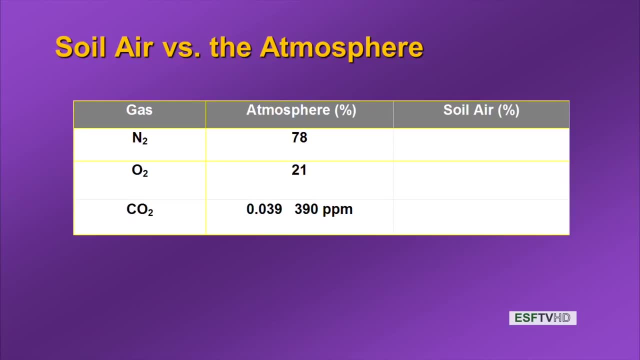 be completely done with soil reaction. That'll kind of push us on to nutrition and that's where we're going. So now we get to soil reaction, Soil atmosphere, soil temperature, and first we talk about aeration. And so to think about 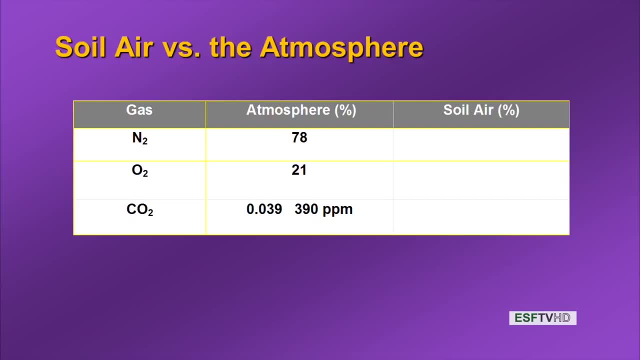 aeration. think about what the soil air composition is, And so we can compare the soil atmosphere with the atmosphere above it And the three major gases- nitrogen, oxygen and CO2, and look at their concentrations here in the atmosphere: Nitrogen, 78%, oxygen, 21% and CO2, about. 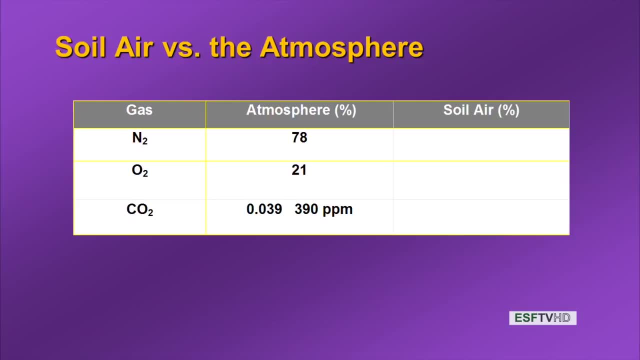 390 parts per million. You also know that, as 0.039%, You should be able to easily convert that right Parts per million from parts per hundred. Well, what are the other gases? Well, there are small gases and there are many. 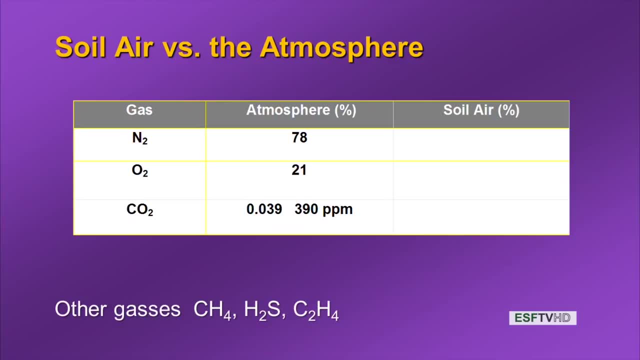 micro-gases, but they're on small concentrations, things like methane and hydrogen sulfide and so forth. But these are in small concentrations and, while they're important from a greenhouse gas point of view, in terms of soil aeration, we focus mostly now on O2 and CO2.. So let's 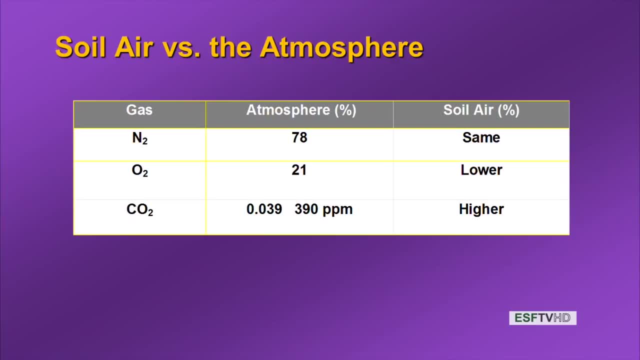 compare the air in the atmosphere to the air in the soil. So if we look at nitrogen, it's about the same, it's about 78%. The oxygen concentration, the partial concentration, partial pressure concentration of oxygen in the soil atmosphere is lower than 21%. Now I'm not going to put an exact number on that yet because there 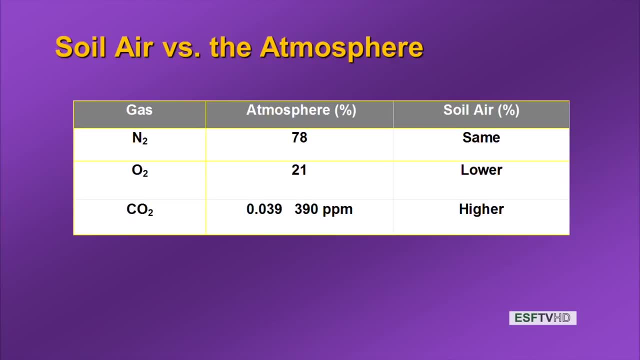 are some factors we'll talk about that influence what that number is: Carbon dioxide. the number in the soil is higher than that in the atmosphere, It's higher than 390, and actually now we're up to 400 parts per million, And so, again, the number is very much dependent on the number of factors. 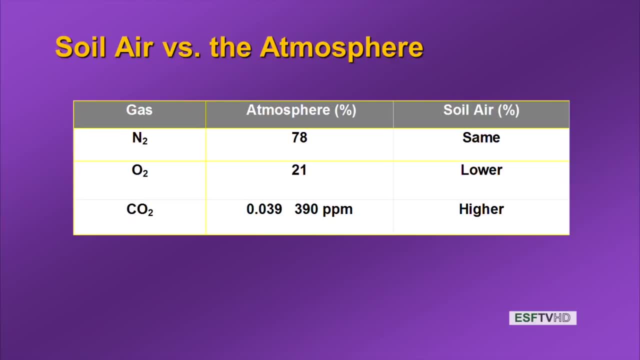 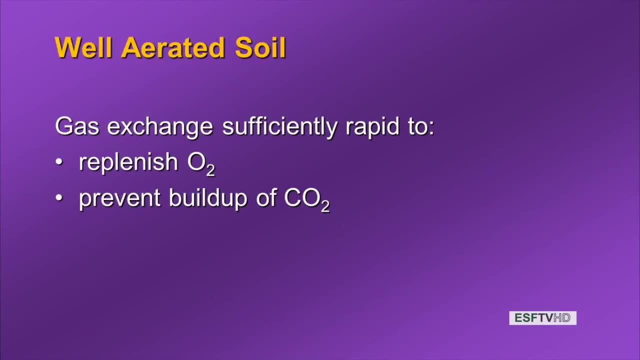 the things that we'll talk about in this lecture. So this sets the stage for us to compare the soil atmosphere with the atmosphere above the soil. So let's think about aeration. We need to define a construct and define this concept of a well. 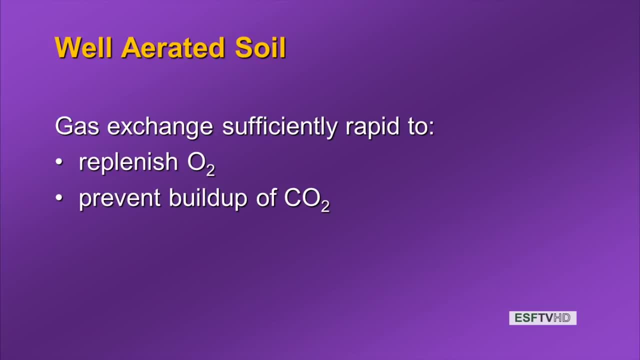 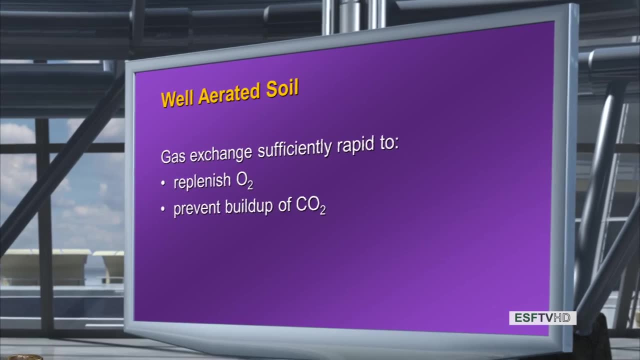 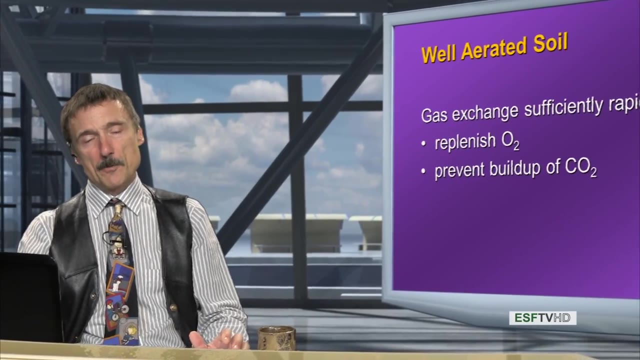 aerated soil. So a well aerated soil is simply one where the gas exchange is rapid enough so that oxygen is replenished And the buildup of CO2 is prevented. So that's our definition: a well aerated soil, gas exchange sufficiently rapid to replenish O2 and to prevent the buildup of CO2.. Very simple definition, And 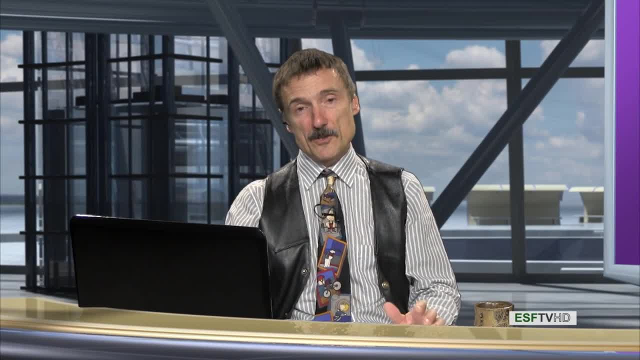 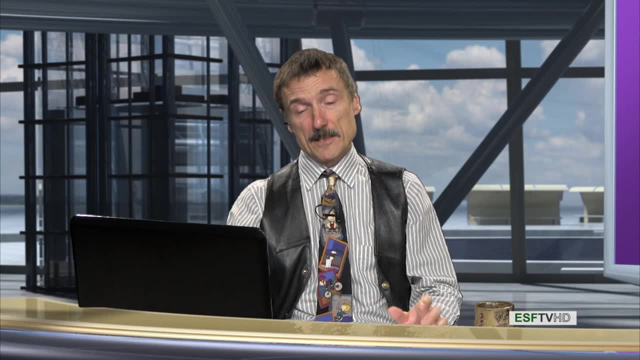 from this definition will flow our understanding of what these soils are, how they're aerated or not aerated. Now this fits in really nicely with physical properties. So this follows well on the heel of physical properties. So let's think about field soil oxygen. 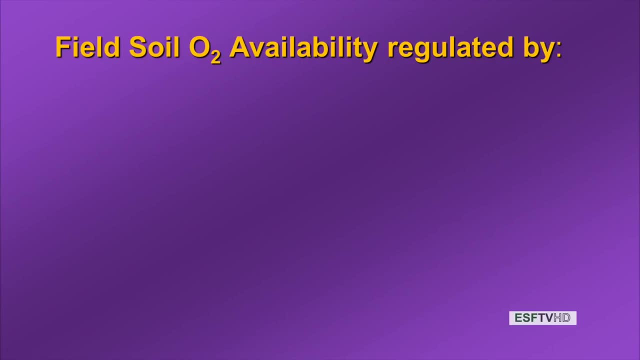 What's happening? What's happening out there? What is the concentration, What regulates it, What constrains the availability? And so we'll look at the number of factors that constrain this availability in the field of Soil, O2.. And the first one, soil macro porosity. And we know macro porosity. we just got completed the soil water. 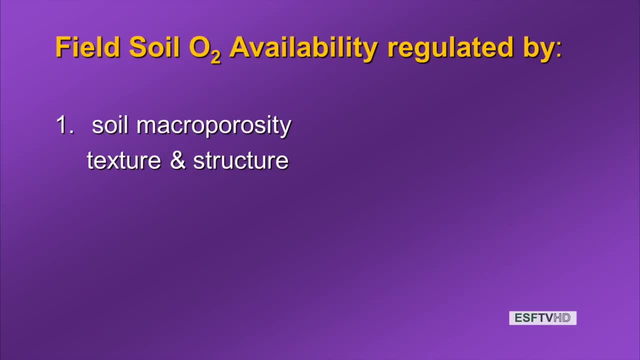 exercise and we actually calculated macro porosity and the soil moisture characteristic allowed that, And now we'll kind of think about that on the other side. So if the macro pores do not hold water, there is our exchange. So soil change will result in what kind of FCs? visit the monsieur, for example. 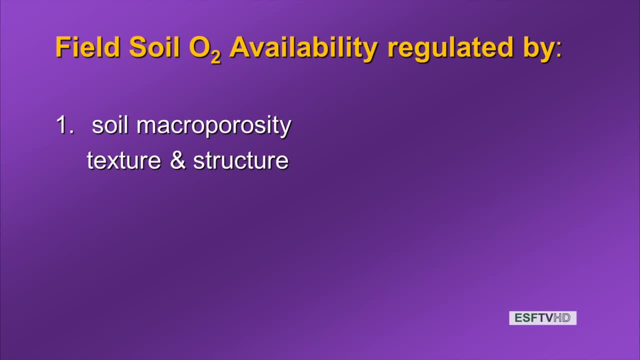 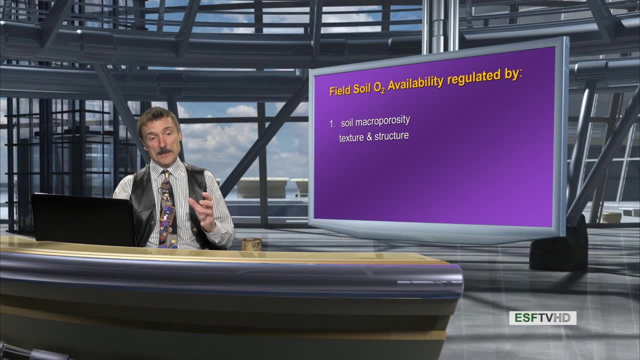 So oiloquits have a ceramic proosity grateful and we go back to physical properties and we're at soil texture and soil structure. Okay, So fundamentally this is a really big piece of big control on this. aeration and oxygen availability is directly related. 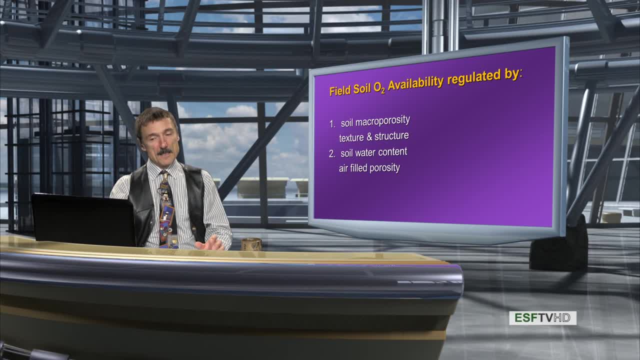 to this. Okay, So that's our first factor. Our second factor is the flip of that right Soil water content. And remember our ideal situation, that Pi shape where we have 50 percent of the pores filled with air, situation, and that P hablarida looks over Lizz and 50 percent of them are level with air. 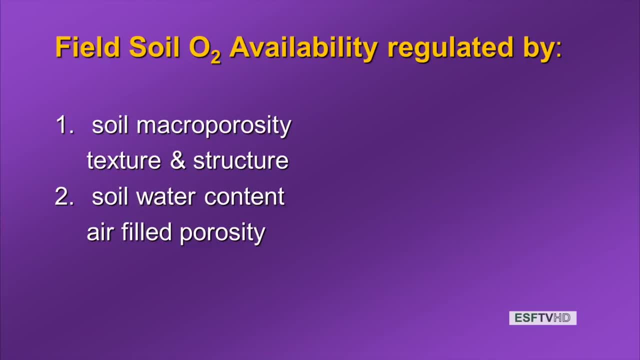 and remember our ideal situation, that pie shape where we have 50 percent of the pores fill with air, being the main answer here. or another ingredient is好了 major part ratio of SMぇ, In addition to fill water content or the air structure that constituents over Lizz. the percentage of sand is lower than NBs. 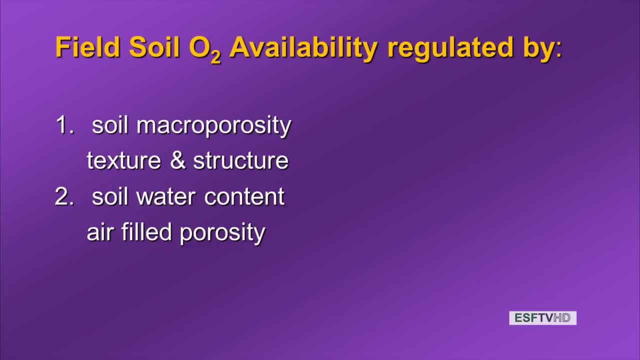 of the pores fill with air, 50% fill with water- macro pores, micro pores- and they are the inverse. So again, a soil pore is either filled with air or it's filled with water. Then we think about air filled porosity, And so those are the 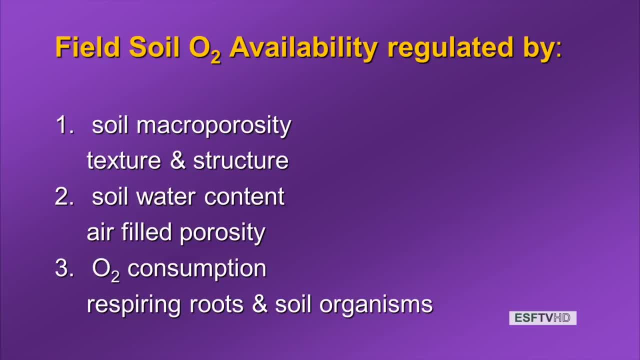 static pieces. Now what's going on? we've got a dynamic system and going on all the same time is the oxygen in those pores and these macro pores, the soil, atmosphere. the oxygen is being consumed. Who consumes it? The roots and the soil. 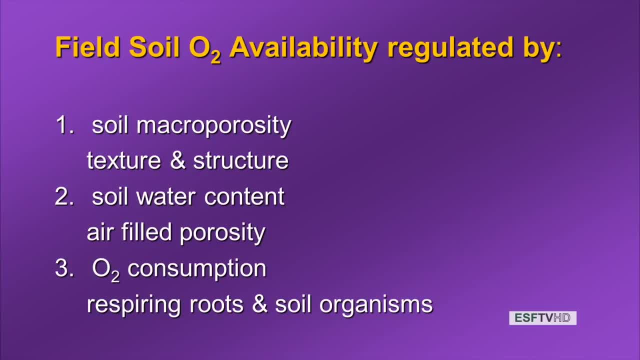 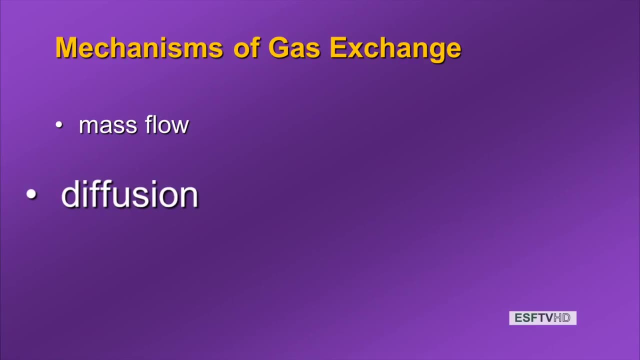 organisms. the aerobic organisms, require oxygen for respiration, And remember that respiration, aerobic respiration, is so much more efficient than anaerobic respiration. How is gas exchanged in those three? So there are two ways we move gas around: mass flow and diffusion, And I have diffusion as the larger one. 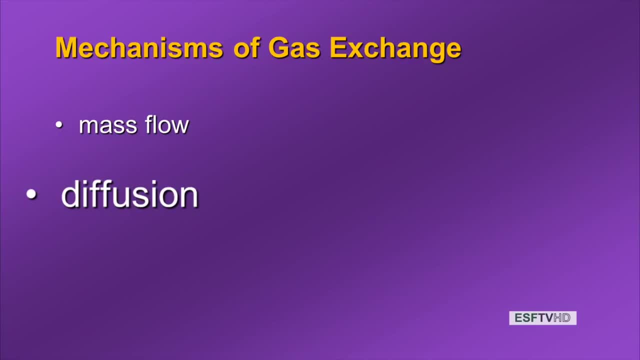 because diffusion is the primary mode that we're talking about for the mechanism of gas exchange in the soil: Mass flow. what is mass flow? Mass flow when wind movement or massive movements of air pressure changes. that's aeration. that's exchange of gas by this physical. 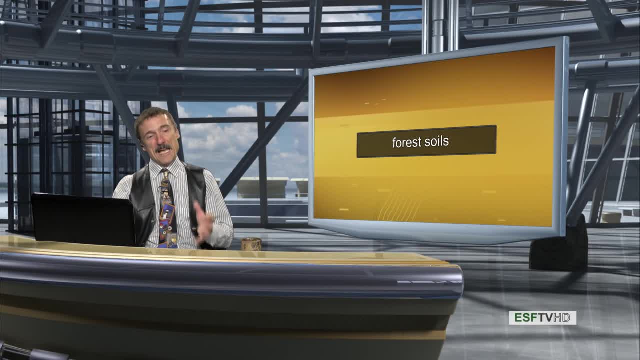 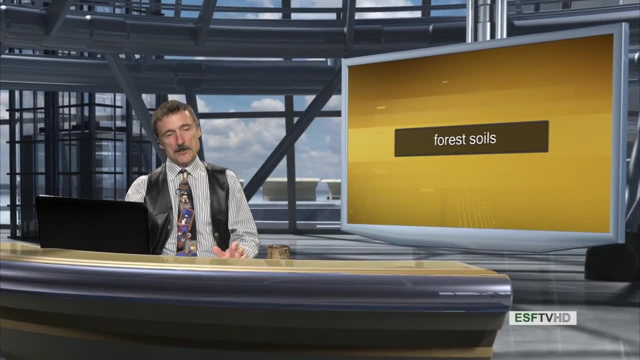 movement. Diffusion is an exchange of gas by action, reaction against the gradient, And so we'll kind of look at that in terms of a picture. What is diffusion? So here's a picture out of the text right. It shows the concept behind diffusion. 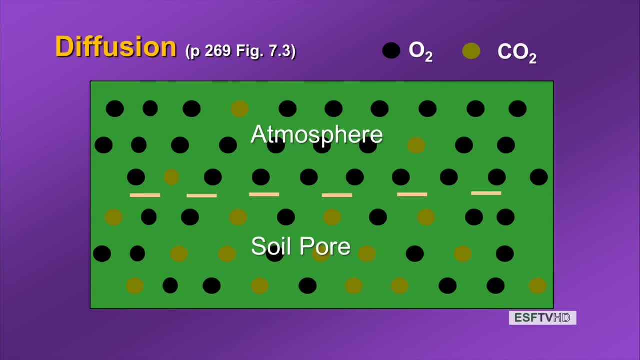 The movement of molecules against the gradient. So we have on top the atmosphere and we have soil pores and here's the soil interface. This dashed line represents the soil And it shows the concentration. So this shows a large number of O2 atoms, gas molecules, and these are a fairly high 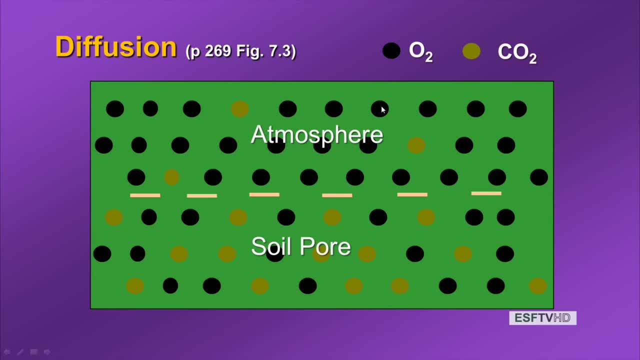 concentration in the atmosphere, and that would be 21%, And this illustrates CO2 partial pressure. this illustrates the number of molecules of CO2, and this is a relative picture. So there are a few CO2's and many O2's. We look down the 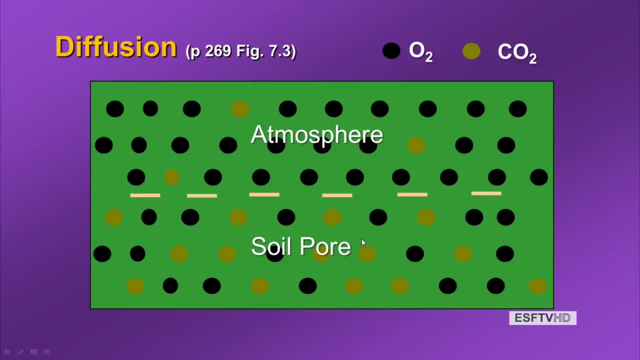 soil and there are many more CO2's and much fewer, many fewer O2's, And so this is a gradient. The gradient flows from high concentration to low concentration, So that's diffusion, And so we have oxygen moving into the soil because the 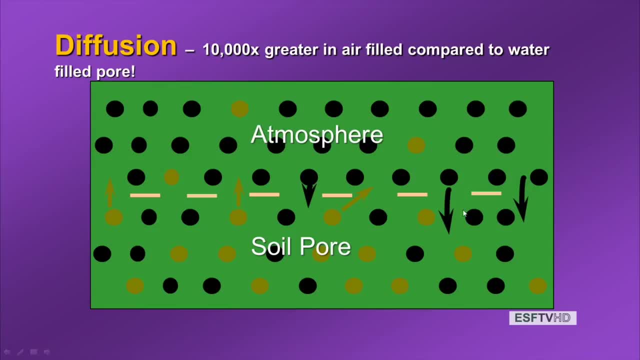 partial pressure, the concentration is greater in the atmosphere moves into the soil. The reverse is true for carbon dioxide. Carbon dioxide concentration in the soil is higher than in the atmosphere, and the gradient is moved to high concentration to low concentration. Soil air is ridding itself of carbon dioxide, And again this 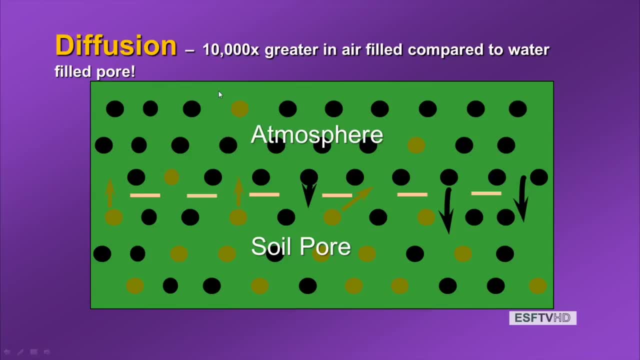 is in response to a gradient, And so this is the process And this happens in air filled pore space. That's why we introduced air filled porosity. And look at the rate: So the rate of diffusion is 10,000 times greater in an air filled pore. 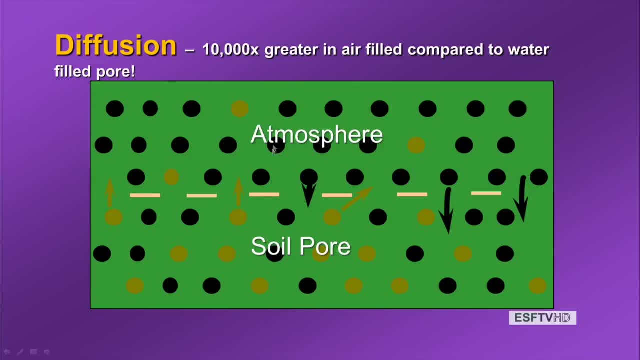 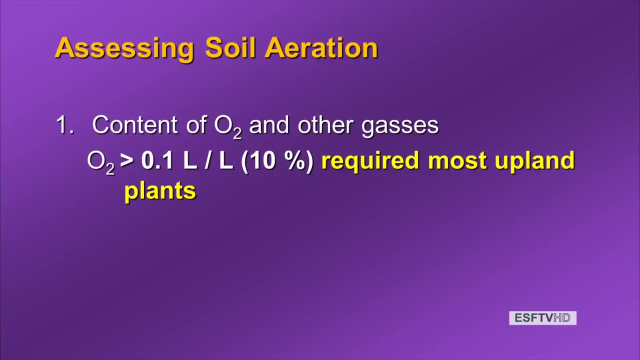 compared to a water filled pore. Essentially, water filled pores restrict this aeration, so we've got to have air filled pores. Brings us back to macro porosity And that's the mechanism. and let's think about assessing it. How would we quantify soil aeration? And there are a number of things we can. 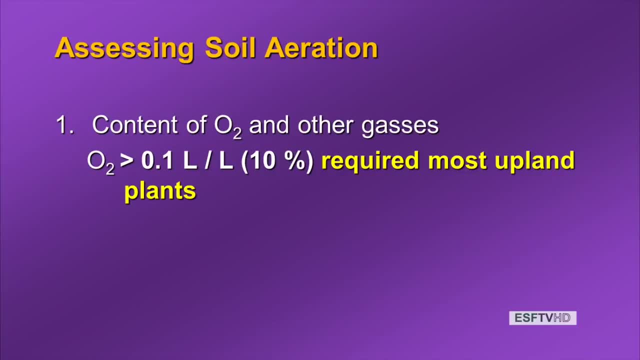 measure to give an indication of soil aeration, And so the first one we'll talk about is the content, concentration of oxygen and other gases in the soil atmosphere. Okay, the number that restricts plant growth in most upland plants, and note that's in. 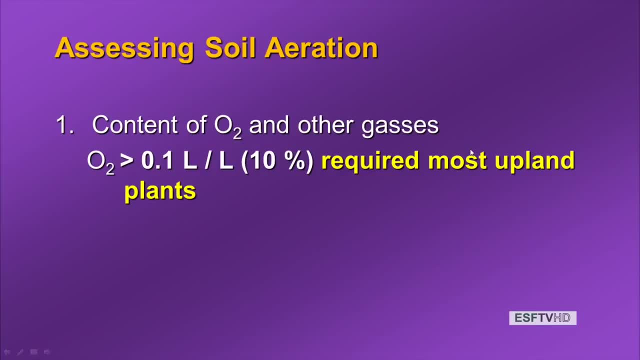 most upland plants there are anaerobic tolerant plants, but for the most part the upland plants. when you get below 10% volume, that is, .1 liter of oxygen per liter of soil, okay, below that number we are in a trouble and plants don't do very well. 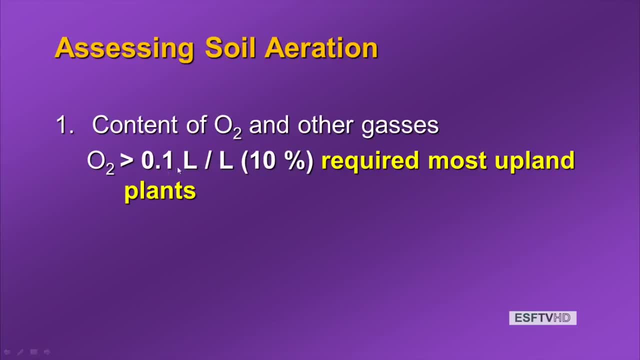 Okay, so that's one way. So a well aerated soil has an oxygen concentration of greater than 10%. okay, so that's a cutoff. That's one measure of aeration. The other side of that is carbon dioxide, So carbon dioxide is the reverse. 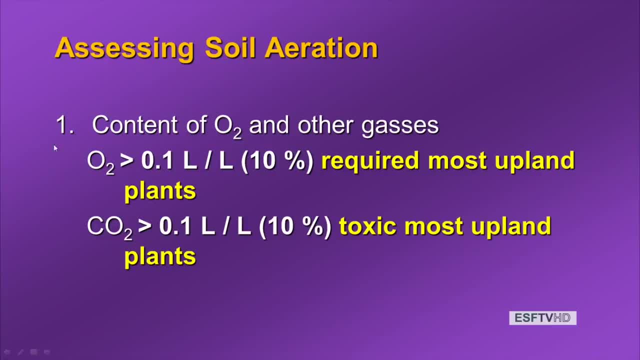 So when carbon dioxide exceeds 10%, it exceeds .1 liter per liter volume of soil, air, soil. this is toxic. Okay. so 10% concentration of CO2 and above, that's toxic. So 10% oxygen too low, less than 10%. 10% oxygen above: too high for CO2.. 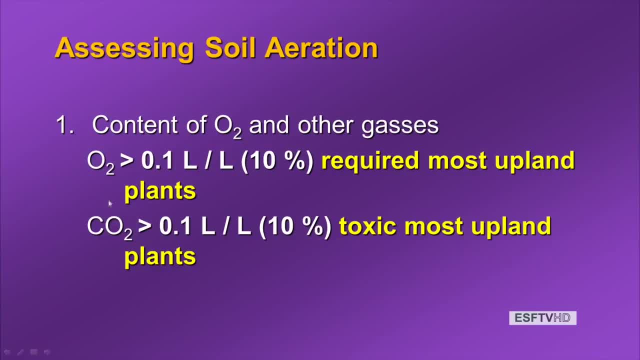 So these are measures, the content of these gases of aeration. So again, thresholds: if you have a concentration of carbon dioxide above CO2, poorly aerated. If you have a concentration of oxygen below 10%, okay, poorly aerated. 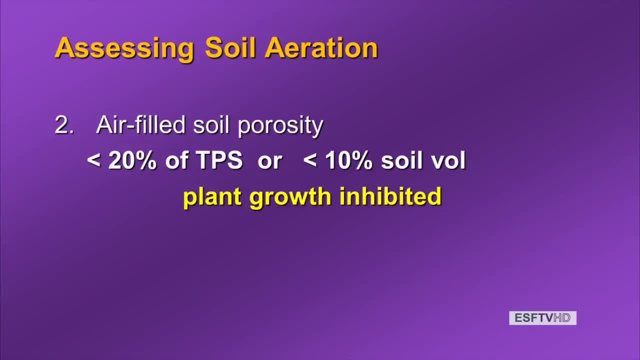 Let's look at another one. Let's look at the air-filled soil porosity. Okay, and this looks pretty close to the volume of soil oxygen filled. And why is that So? air-filled soil porosity: less than 20% of the total pore space air-filled, okay. 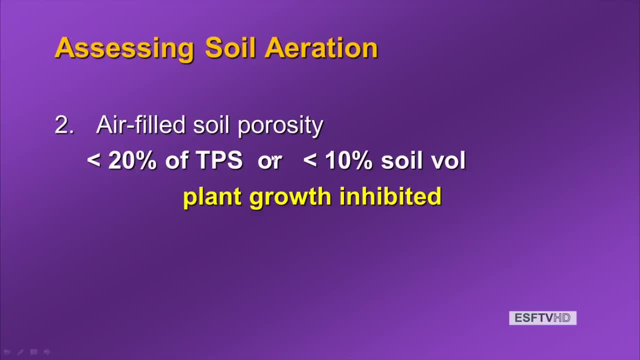 that reflects a problem. okay, less than 10% of soil volume. And why is that? This should be familiar If we think back to our diagram of the soil, the ideal soil having 50% pores, half of those pores filled with water, half of those filled with air. 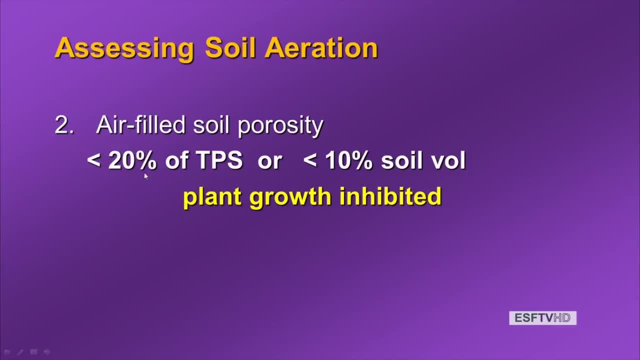 So if we think about this as total pore space, Okay, And if 20% less than 20% total pore space is in trouble and if half of those are air-filled and half are water-filled, that's where this 10% comes from. 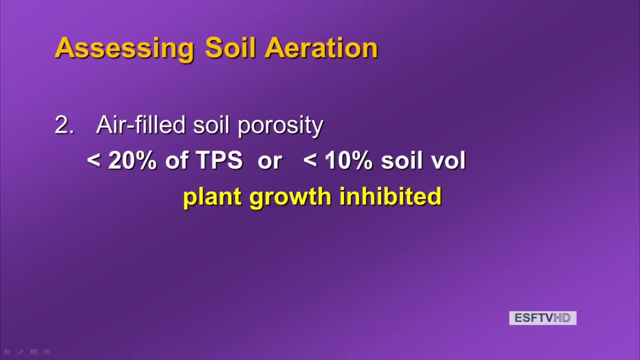 So this is a threshold back of the envelope calculation for aeration. If you have a soil with less than 20% air-filled pore space, you're likely to have a poorly aerated soil. Or you can express that in terms of the soil volume, because about half of those would 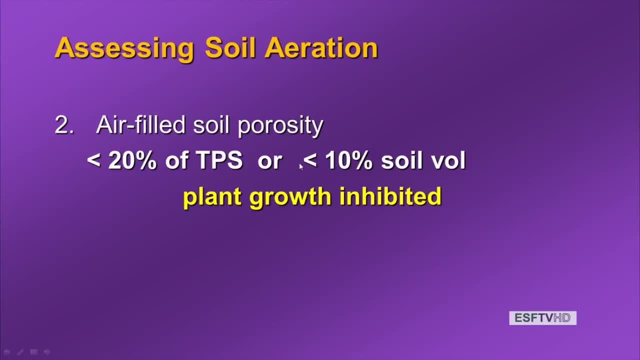 be micropores in the average sense. that would be bad. So plant growth is inhibited. So now we have two things: We have concentrations of carbon dioxide and oxygen and we have this air-filled soil porosity, two variables we can measure as an indicator of soil aeration. 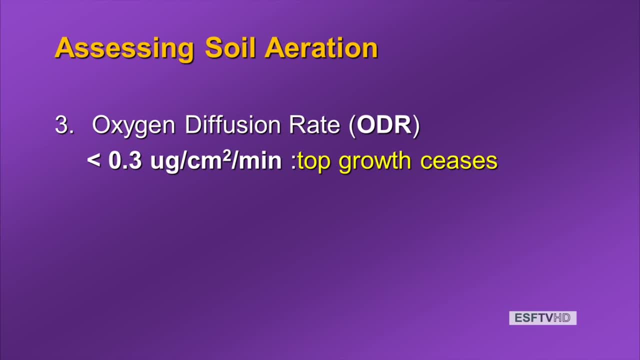 But there are more, Okay, And so we'll go through them. We can also look at the rate of oxygen diffusion and the so-called titled the oxygen diffusion rate, ODR oxygen diffusion rate, And here's the number. here's the threshold where top growth ceases: three-tenths of a. 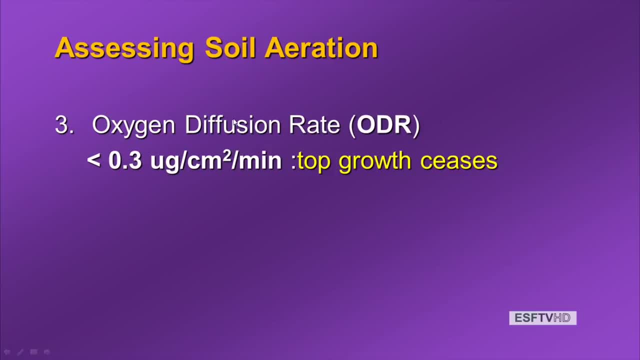 microgram per centimeter per second, A unit area between the top growth and the top growth ceases. So this is a diffusion rate. It is an amount, microgram, a unit area, centimeter squared per unit time. It's a rate of movement of a certain amount of gas over a certain area, over a certain 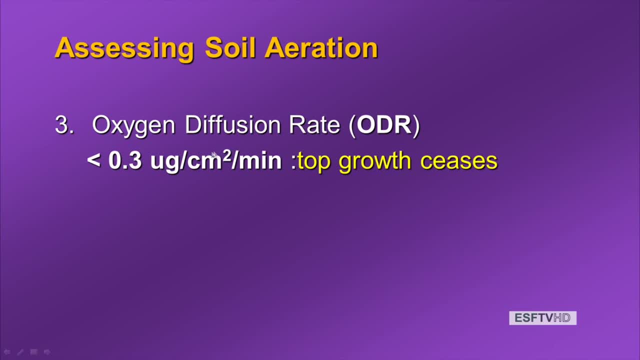 time period. So when you get below three-tenths of a microgram per centimeter per second- sorry per minute- top growth ceases. So here's another measure of a poorly aerated soil. So poorly aerated soil is one. 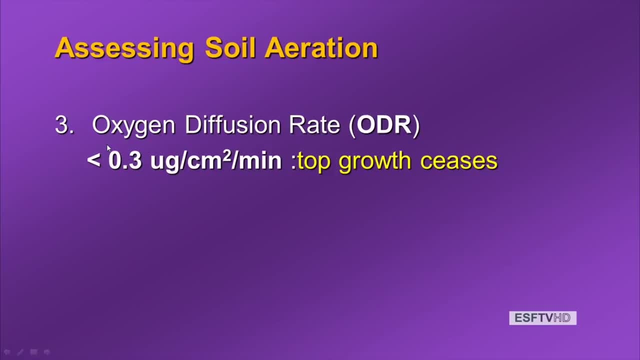 It's the amount of oxygen that's released from the top growth, and the top growth that's which has an oxygen diffusion rate less than 3 tenths of a microgram per centimeter squared per minute. Okay, that's three. We can also consider root growth. 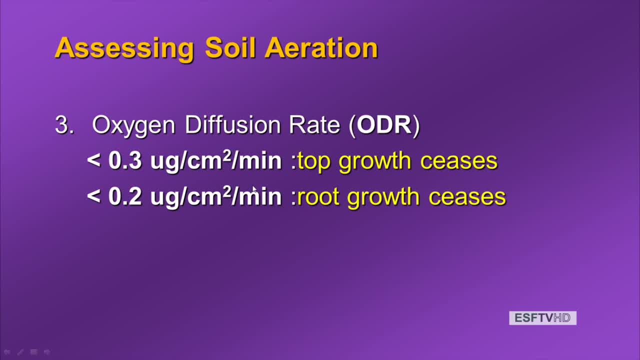 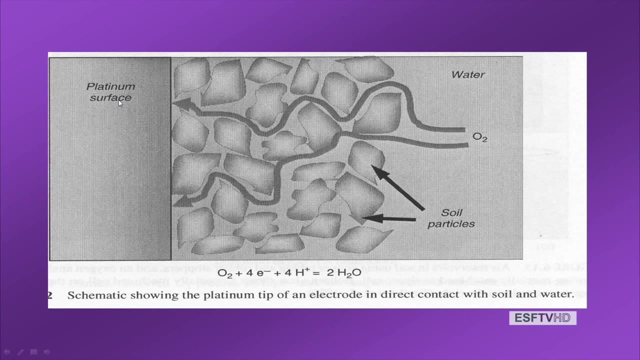 And root growth is pretty close. You know it's .2 micrograms per centimeter squared per minute. So you're in this range and you're going to lose growth. enough said, How do you measure oxygen diffusion rate? Well, we can use it on a platinum surface and with a little bit of electricity. 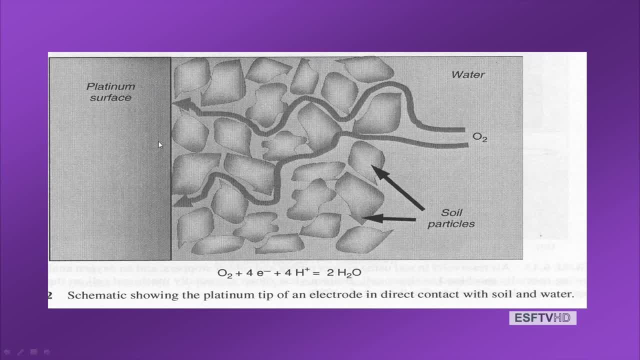 And so the rate. we and these are actually pretty tricky to do- to get these in the soil because these are influenced by pH and it's a tricky measurement But nevertheless you can insert these platinum electrodes and measure the rate of oxygen diffusion. 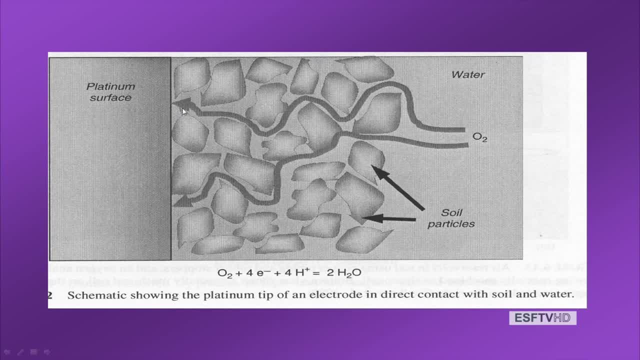 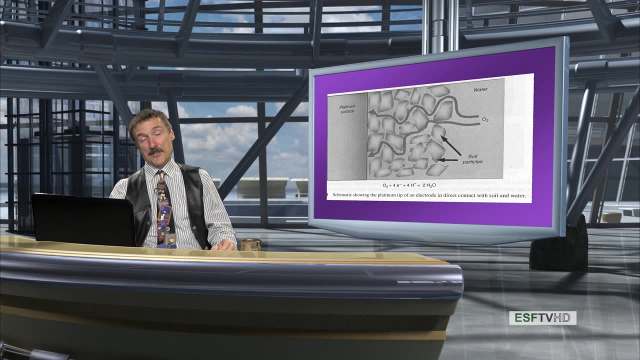 And the rate of diffusion will change electrical conductivity across it and you can translate that into a measurement of diffusion. Okay, So that gives us another way. So now we're looking at gas concentration, We're looking at volume and diffusion rate. So we have three different numbers, three different variables to assess aeration. 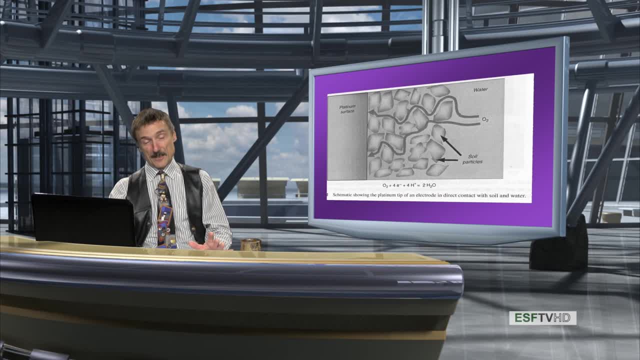 And so I'm going to ask you to know these, because this will be a key to understanding or expressing, or quantifying diffusion. And again, this is part of productivity: aeration: a well aerated soil is going to contribute to our concept of productivity. 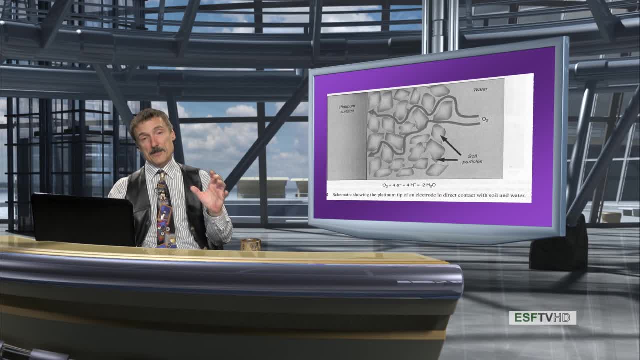 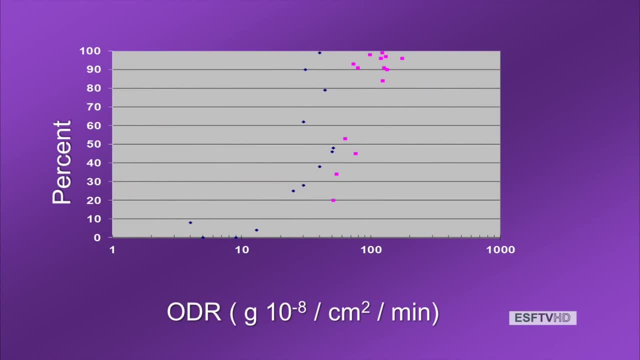 And we're building on soil- physical productivity. We're building on soil- physical properties. So these numbers, this set of numbers, these thresholds, should be committed to memory. What does some data so? I have a colleague at University of Georgia that has a couple. 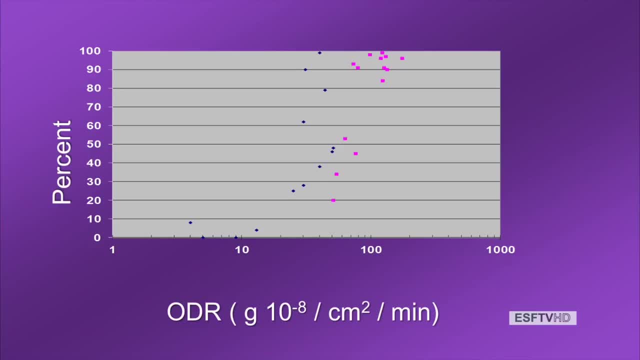 of grad students that tried to assess aeration for a couple of systems. okay, And this graph here, okay, shows a percent response either to root or biomass. okay, And this shows oxygen diffusion rate and this is grams 10 to the minus 8 per centimeter. 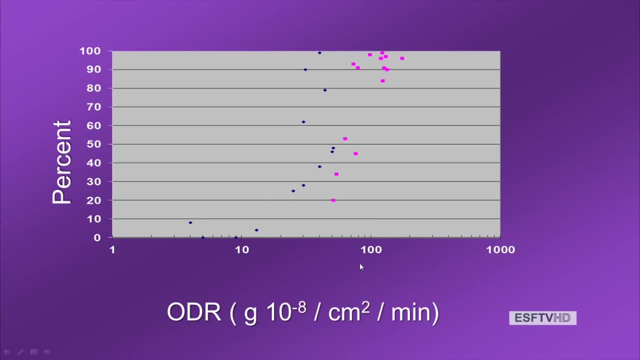 square per minute. okay, Note the log scale. And there are two systems here. okay, loblolly pine seedling emergence. okay, And that's represented by these orange, I guess these pink squares, And it's pretty linear related. 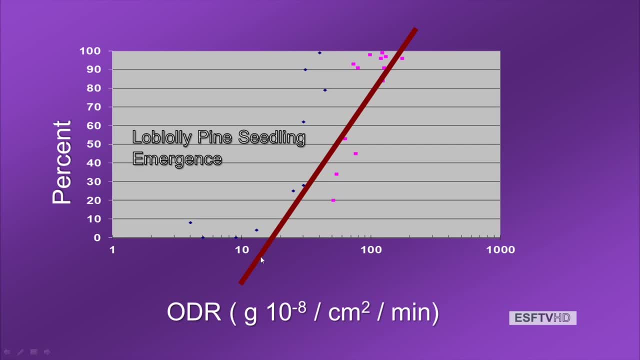 So once you get below, get below a very small number, look down here around 10,, 12,, 0, you're getting to a essentially no response. So if you look at the response percent of loblolly seedling emergence, it's 0 around. 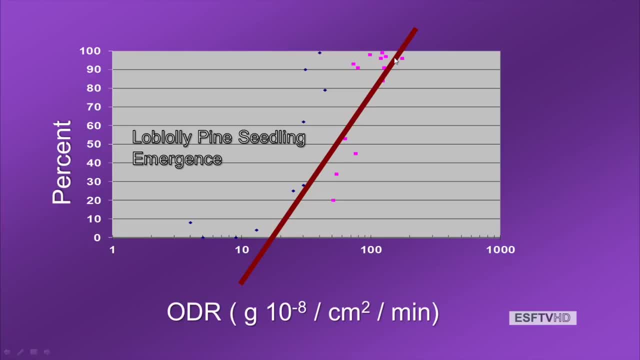 here, And if the oxygen diffusion rate goes up, the success or the response of those seedlings goes up. So that's quite an interesting system and one way to look at that. okay, We can look at another system, a totally different system, and look at that in terms of cotton. 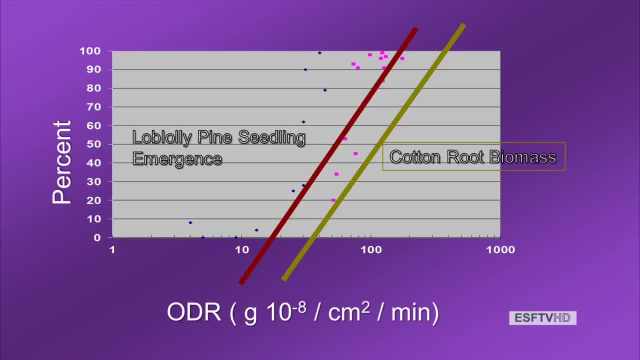 root biomass and the same kind of thing. So cotton root biomass expressed by these wonderful, wonderful blue diagrams, and you see the same. actually this line should have been over here. somehow I stuck that line over here. At any rate, it's the same linear. 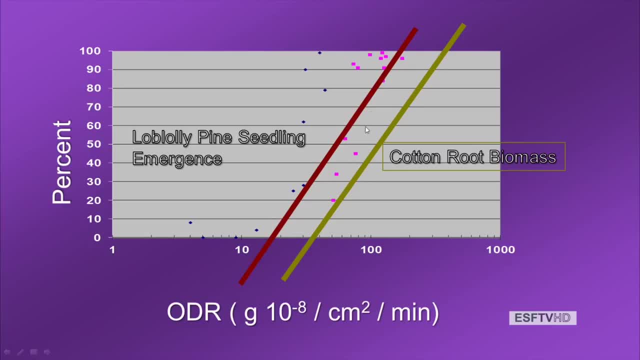 It's the same linear relationship, so the slope is about the same right And this again shows the linear relationship of a totally different system. The cotton root biomass increases as the oxygen diffusion rate increases. So both of these are indoor pot studies and lab studies, but they show the importance. 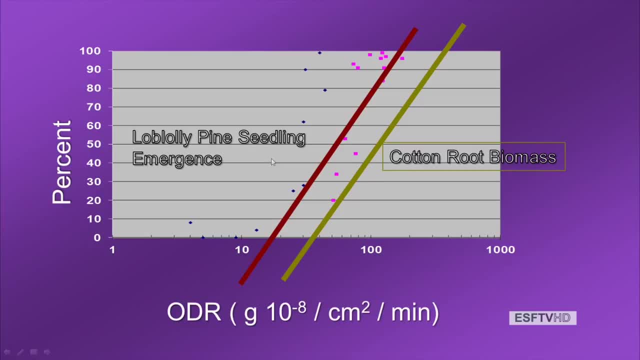 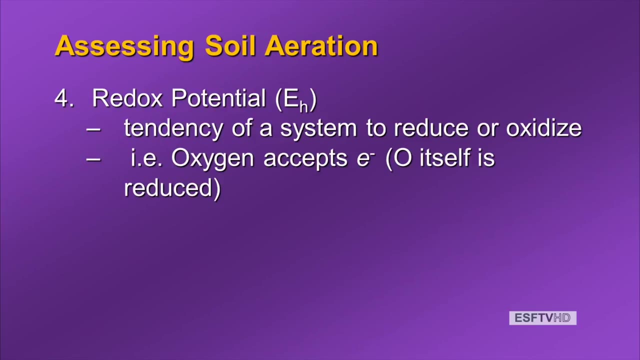 of oxygen diffusion rate relative to productivity, whether you measure it in seedling emergence or whether you measure it in cotton root biomass. Okay, so there's a fourth way and we can actually measure the redox potential, the oxidation reduction potential, and this is called EH. okay, capital E, small h. 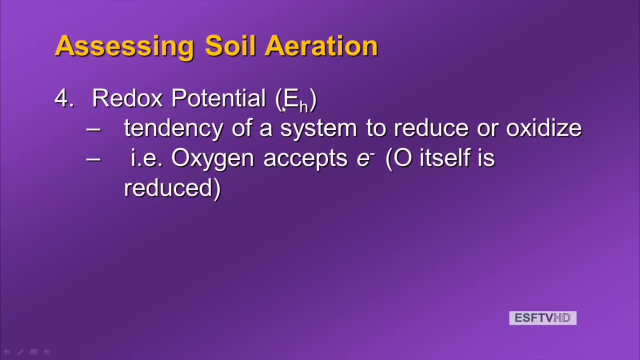 And this is a number. it's measured in volts or millivolts. that expresses the tendency of a system to reduce or oxidize, hence the term redox potential. and again potential. it's measured in volts. And so how does that work? 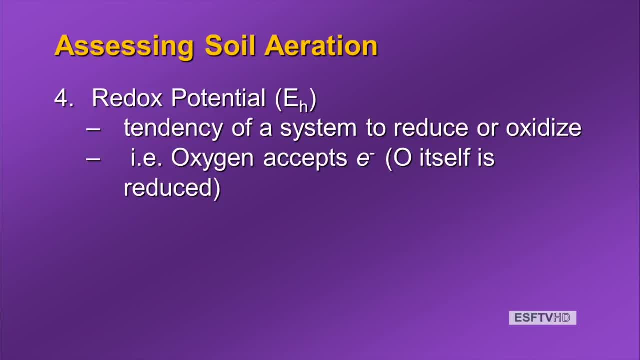 Oxygen accepts electrons- Okay- And oxygen, and so it's becoming reduced. So when this occurs, we can measure this, the change in voltage, we can measure this potential- okay- and describe that as the tendency to reduce or oxidize. 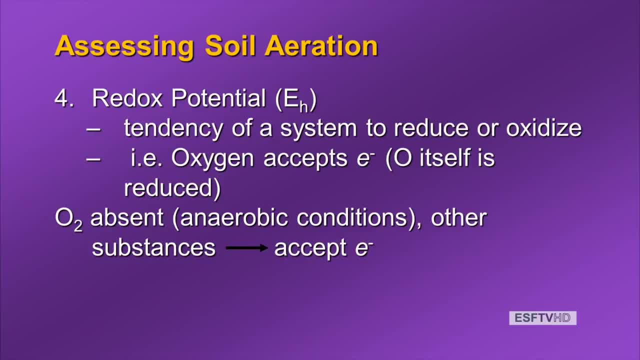 What's the reaction? okay, O2 production, O2 absent. So when O2 is around, the system will oxidize. there's plenty of oxygen. oxygen happily accepts electrons. okay. What happens when oxygen is depleted? In that case, something else has to accept the electrons. okay, something else and this: 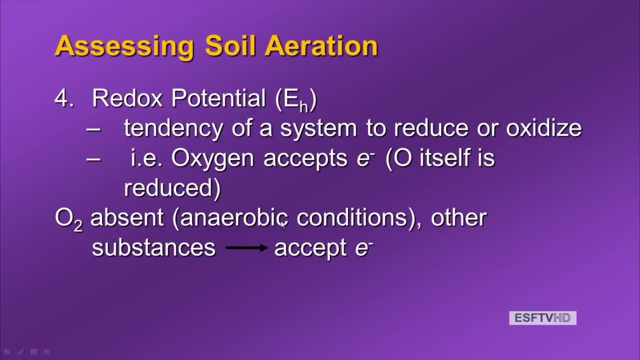 is the absence of oxygen is called anaerobic conditions. okay, poorly drained conditions lead to absence of oxygen and other substances accept electrons. Where do the electrons come from? Respiration. So, even in aerobic systems. not even in, but in aerobic and anaerobic systems, the biota. 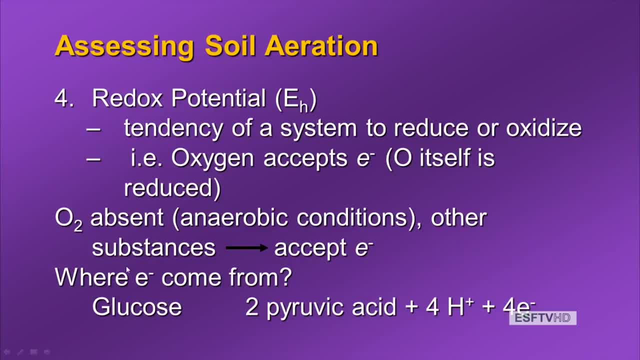 are producing. As long as you have oxygen around, respiration kind of proceeds unimpeded. But when the oxygen goes away or becomes limiting, anaerobic respiration stops and anaerobic respiration goes on. So glucose is broken down, remember, with glycolysis. and if you took some chemistry, organic chemistry, 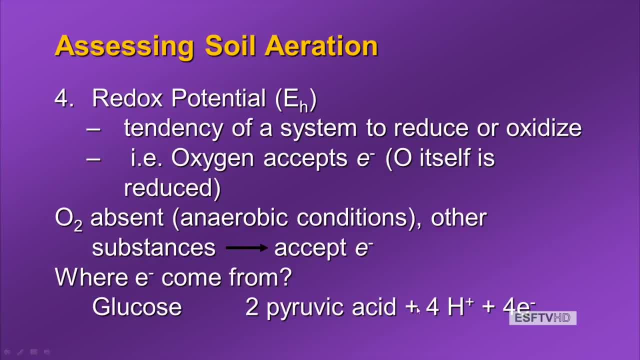 biochemistry. this produces energy and it's broken down to pyruvic acid and hydrogens. But one of the things in breaking this down, this is the beginning of an electron chain. Okay, The electrons have to go somewhere or else the process stops. 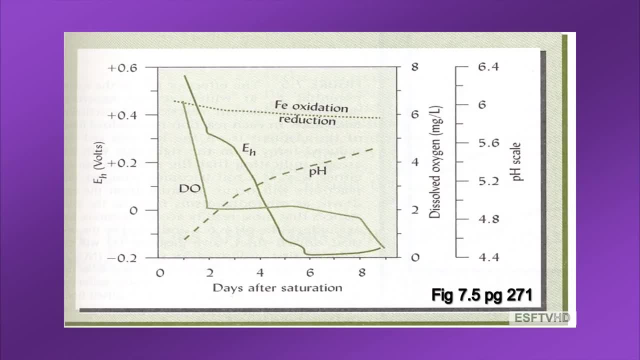 They transfer down the chain. So let's look at what happens with this redox potential. So here we have a graph- and this is out of the text, figure 7-5, and it shows electron redox potential, EH, and this is measured in volts, okay, and it goes 0 to .6, okay. 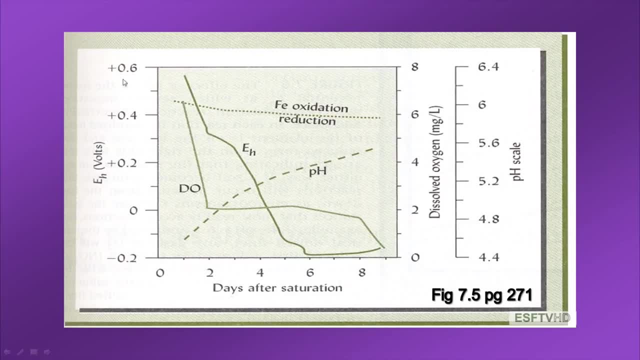 you could express these in millivolts by multiplying by 100, by 1,000,. okay, and note what happens. this is days after saturation, okay. So what happens after you saturate a soil? okay, all of a sudden, immediately, what happens? 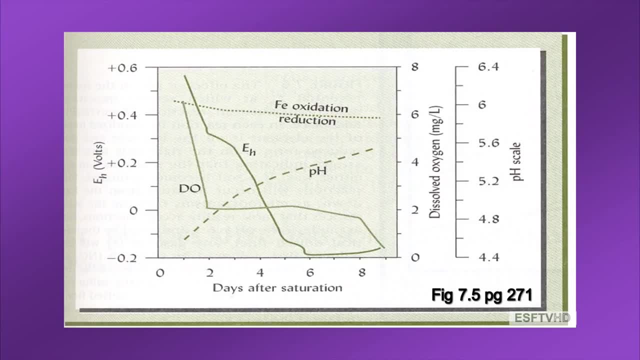 is the plants and microbes. they take up all the dissolved oxygen and it drops tremendously. So here we saturate, okay, and we're looking at DO for dissolved oxygen. okay, and the dissolved oxygen is showing over here on the right. okay, and it's milligrams per liter. 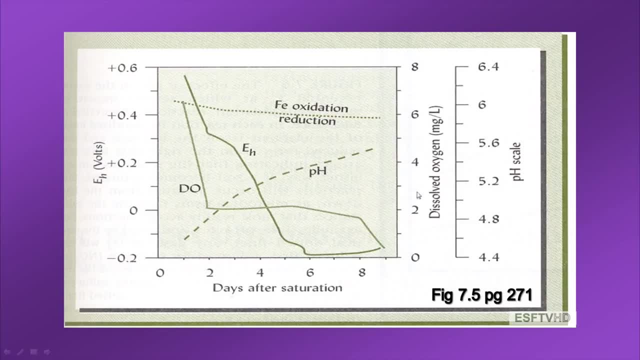 and over here on the far right is the pH scale. So note what happens to this dissolved oxygen. it drops precipitously from about 6 milligrams per liter As the plants and then it's kind of stabilizes because there's pretty much none left. it's. 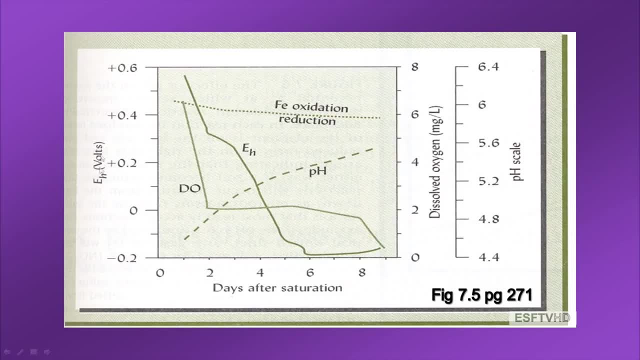 depleted. okay, and what happens to the EH? the EH, the potential, drops precipitously- So well aerated soil, high EH .4, and then, as the oxygen is depleted, the EH drops very low to zero and even goes negative. okay. 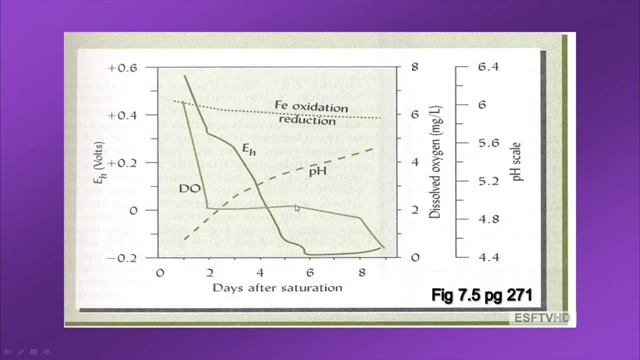 And if you look at that, that's pretty highly correlated with dissolved oxygen, okay, and everything below this line. This line is anaerobic and it's called reduction, So iron is oxidized below this line. So as soon as oxygen is depleted, okay, iron is reduced. 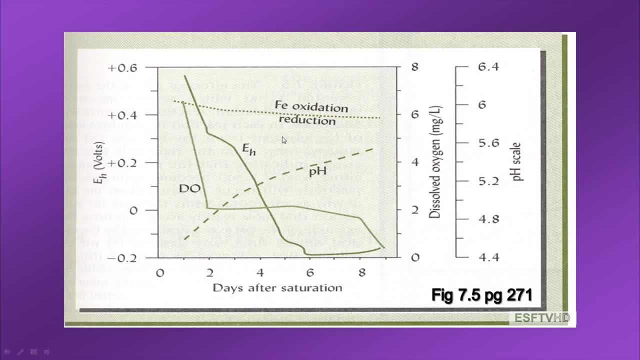 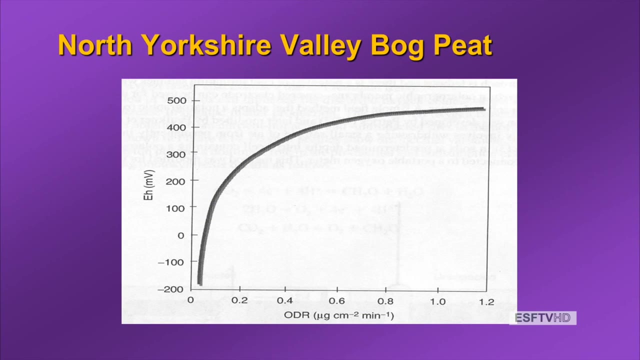 Iron is now getting the electrons that oxygen would be, but there's no oxygen to get the electrons. At the same time, notice that the pH goes up. okay, So this will come into play later. the pH goes up. Here's some data from the North Yorkshire Valley. 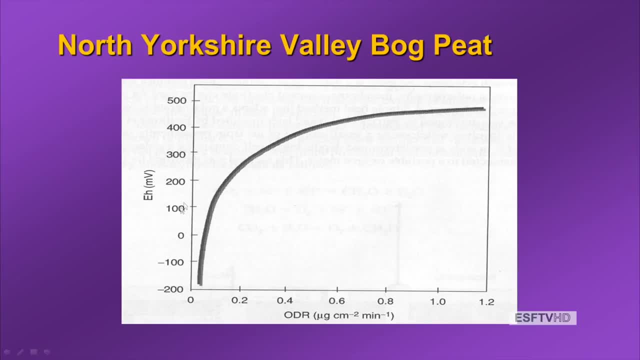 Yorkshire Valley peat bog and shows very similar things, some data that shows EH and ODR. So these things are related. So we've measured the aeration, We've kind of expressed that with several variables. We've expressed it with electron, with this potential, with EH. 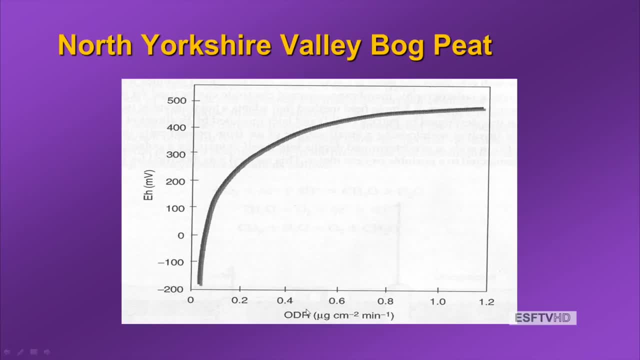 We've expressed it with ODR, We also expressed it with total porosity And, as you might expect, all these things kind of flow together. So if you look at EH And you look at the oxygen diffusion rate, they're pretty highly correlated. 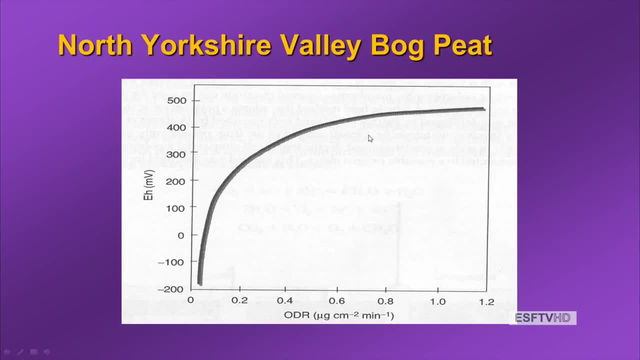 And so as the EH increases, you get more positive. okay, The oxygen diffusion rate increases. And remember where the problem area is. it's around 0.2 to 0.3 micrograms per centimeter square per minute. So right around here, okay. 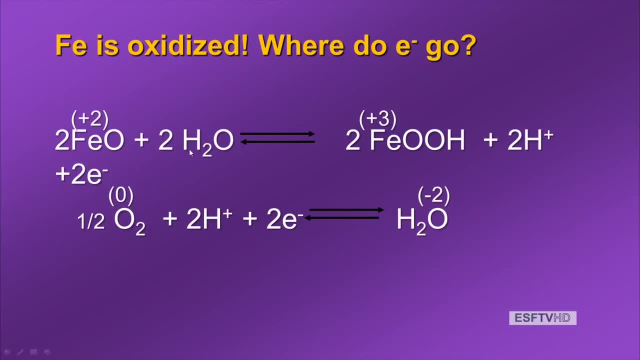 So what's happening with this system? So we've got iron, now getting the electrons, So let's take a look at this, Okay, So here's iron plus 2, okay, and in water, And we go to iron plus 3.. 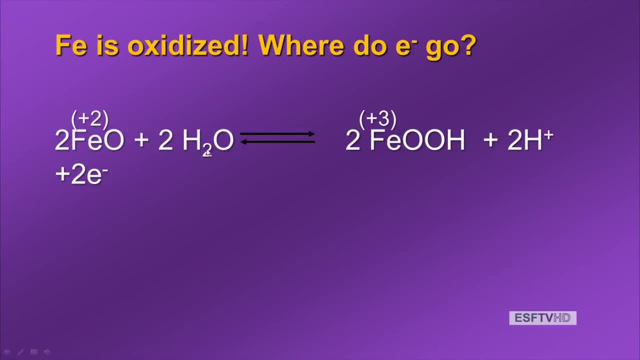 So this is oxidation or is it reduction? You go from plus 2 to plus 3.. That's oxidation, okay. So these electrons go to iron. So iron is getting electrons. Next up on the ticket, we look at oxygen in the system. 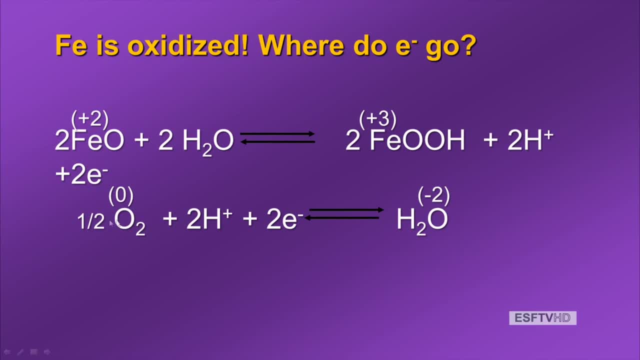 So we add oxygen in. okay, So oxygen receives the electrons. So if oxygen is getting electrons, okay, this is reduced to water, and this is what the system looks like. The electrons are going to oxygen, So oxygen is getting reduced, okay. 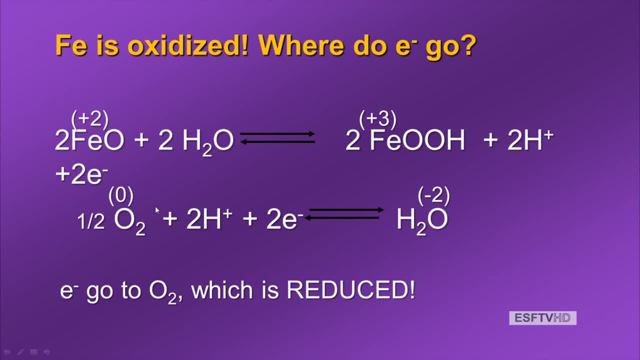 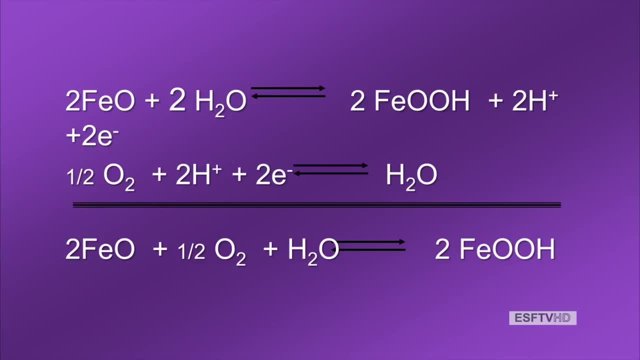 So plenty of oxygen around The system is oxidizing, But oxygen itself is reduced. Let's put those two together. And if we have FeO and we go to FeOOH and we add in the oxygen, here we go to FeO and 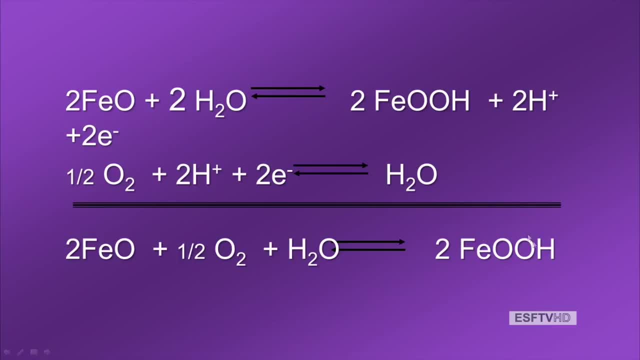 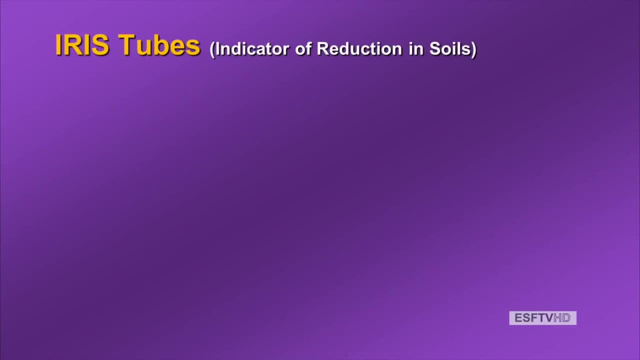 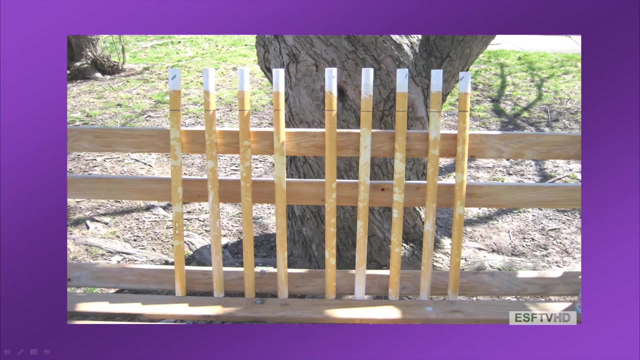 a half of oxygen and we oxidize that to FeOOH. okay, What's another way to measure aeration? This is a clever thing called IRIS tubes, and IRIS stands for Indicator of Reduction in Soils. okay, So these are tubes and they're painted with an iron oxide. okay. 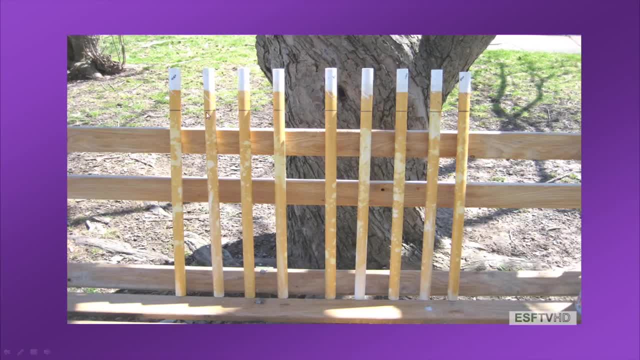 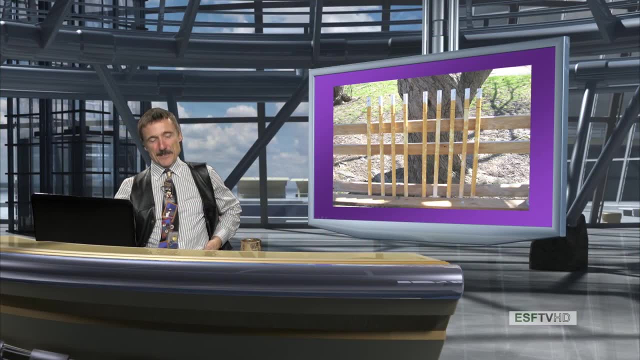 And when you put these in soils, okay and they're reduced. that gets rid of the iron, So these are pretty neat. So this was developed by some colleagues down at Maryland and thought that it would be an easy way to look at oxidation and reduction. 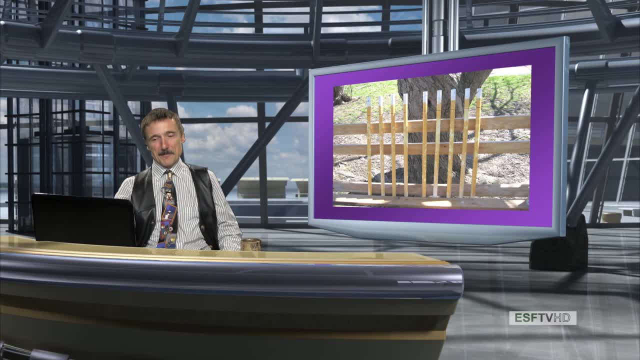 So if you reduce iron and peel it off, you'll kind of make it disappear. This is an iron paint, right? And if you put this in a reduced state it's going to get oxidized. And if you put this in a reducing system, it will be peeled off and it will undergo. 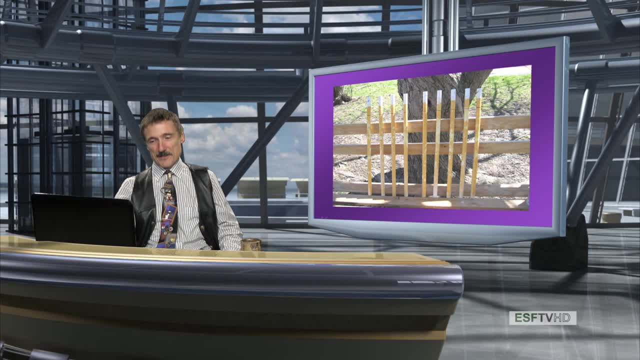 this reaction and become soluble and be reduced, And this is a visual picture of reduction. That's pretty cool, That's pretty cool. And then you can get a little bit more- let's say, clever and you can actually measure the relative area of these with some sensing, some camera sensing, and then get an index. 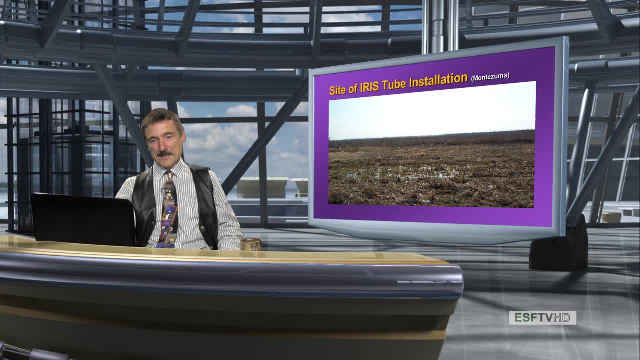 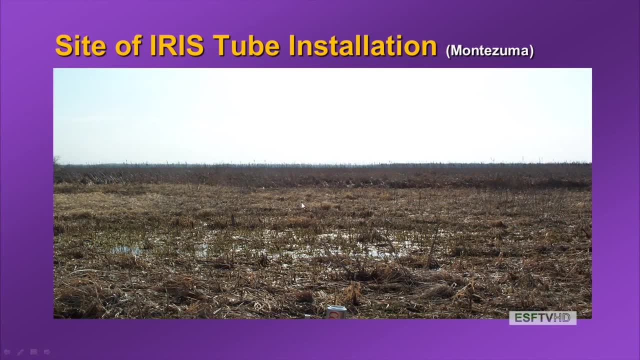 of reduction, So this was done. So here's a site at Montezuma. This is the site of the wetland meeting about four or five years ago And this, of course, you can see this is a poorly drained site. It's flat. 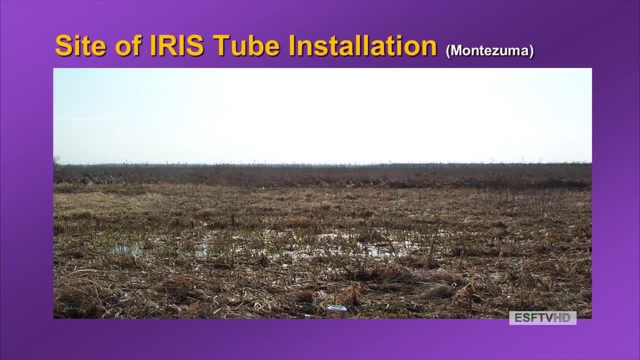 It's anaerobic, It's a wetland And there's clearly reduction going on here. So these tubes were installed and those tubes that you just saw before went into this site, And the result of this is that iron is reduced. 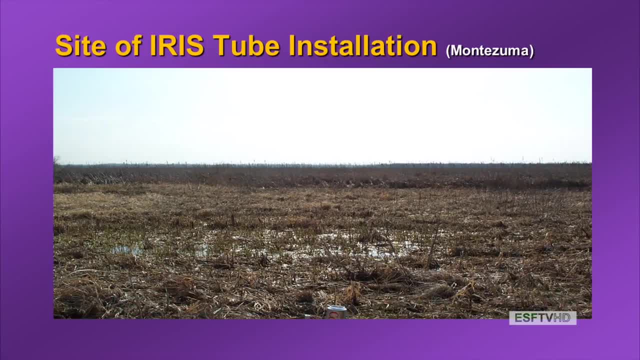 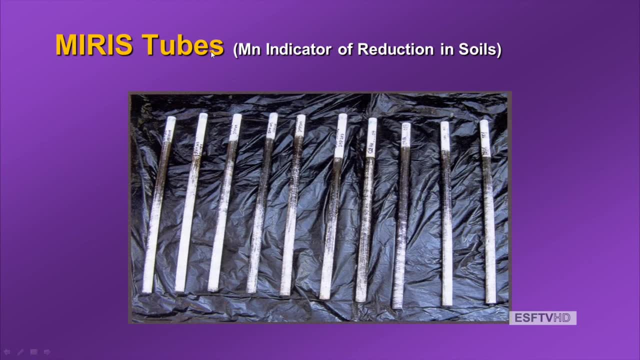 It then doesn't stick, The paint peels off and you have an indicator of reduction, the iris tubes. You can do the same thing with manganese, OK, So manganese also can be reduced, except electrons, And this is what manganese. manganese coatings are black. 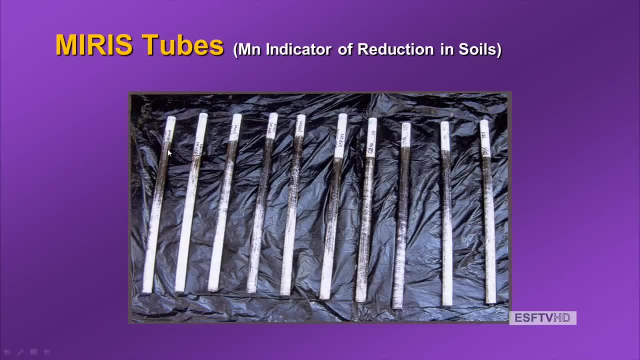 And you can see what happens to these manganese coatings. These start out with a real painted black all the way down the manganese coating And you look at this and all this manganese is gone. This occurs in a very short time. So this is the visual manifestation of reduction by the fact that this reduced manganese peels. 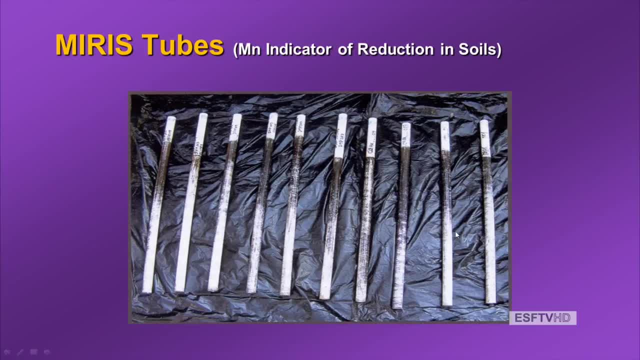 off and dissipates from this painted PVC. So again, another very clever thing, these miras tubes for manganese and iris tubes for iron, And we go back and remind you that these were placed in this situation. These were placed in the situation of that picture from Montezuma, this wetland. 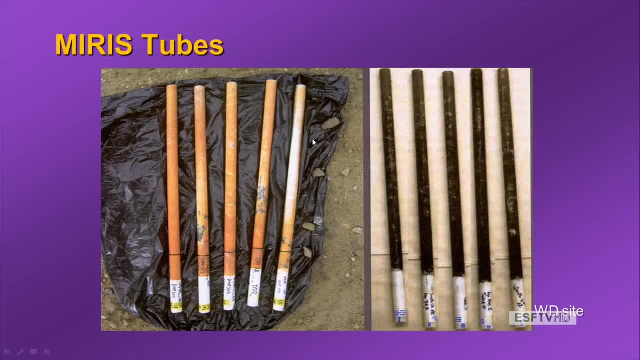 Here, side by side, the miras tubes and the iris tubes. OK, So if we go to a well-drained site, look at the difference. OK, There's plenty of oxidation, Manganese isn't reduced, And what a nice change, right? 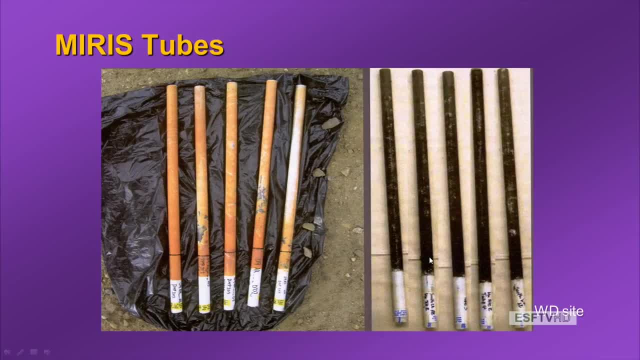 You have these beautiful manganese coatings that stay. So that's a contrast. So the difference between this and the previous slide with all this white exposed, white where manganese reduced, manganese dissipated or left the PVC. again a visual picture of reduction. 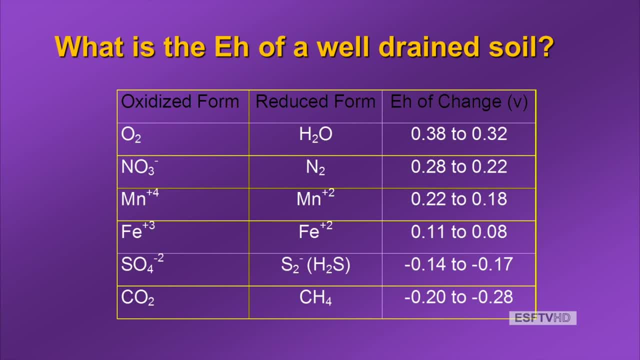 OK, So let's tie this back again to our EH value, And we showed you a slide showing about 0.4 when we had no problem with dissolved oxygen, And then this went down from there. So here's the EH slide of, and we'll go down and look at the elements that accept electrons. 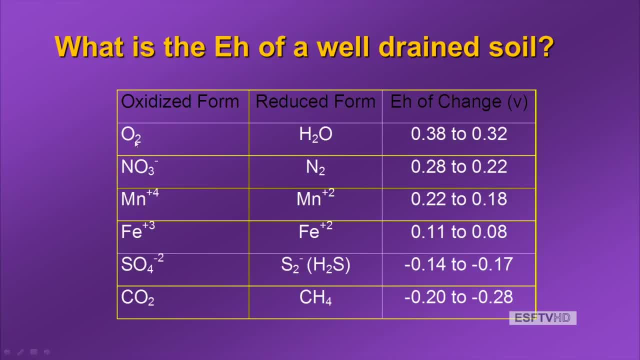 as they're depleted. So we'll start with oxygen. OK, This is the oxidized form. This is the ultimate electron acceptor in a well-drained system. OK, When oxygen accepts those electrons- I showed you the slide before That- it is reduced to water. 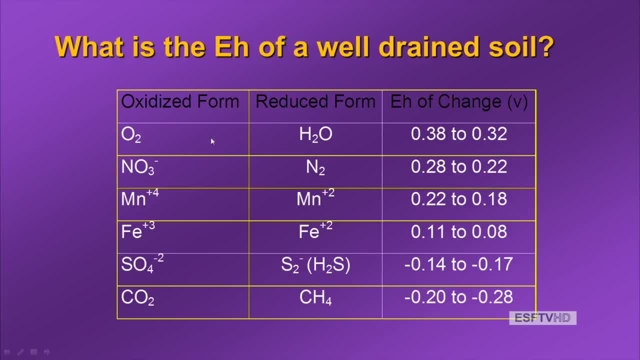 So oxygen converted to water. Now, when we're starting to deplete oxygen, OK, and this starts to run its course, the EH changes from about 0.38 to 0.32.. So, as you're depleting oxygen, EH is dropping. 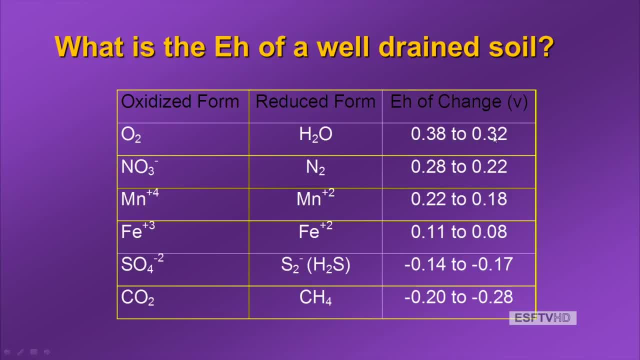 OK, It's dropping from 0.38 to 0.32.. Now, eventually, all that dissolved oxygen dissipates. It's all reduced. What happens next? The next thing in line to receive electrons is nitrogen Nitrate, NO3 minus. 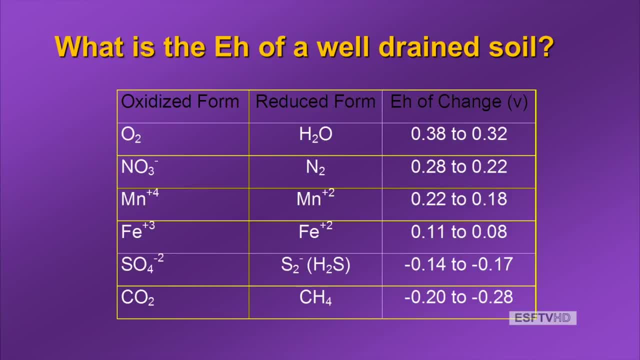 OK. NO3 minus begins receiving electrons. There's no oxygen left, So nitrate starts to receive electrons. Nitrate is reduced to nitrogen gas N2.. And this occurs in the range of the EH of 0.28 to 0.22.. 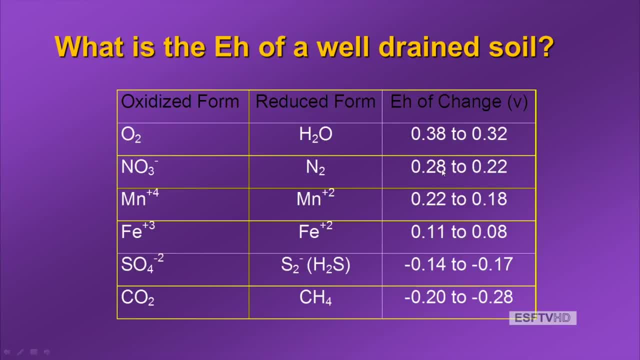 OK, And these are volts, Right. Eventually all the nitrate is reduced And when all that is gone from the system and you still have anaerobic respirations, the electrons need to go somewhere. And the next thing in line to receive it in terms of the electromagnetic spectrum. 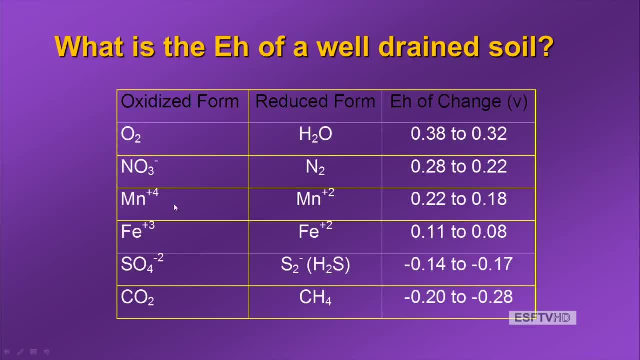 is manganese plus 4.. OK, Manganese plus 4 is then reduced to manganese plus 2.. OK, You're decreasing balance, You're reducing The EH value of this change. when this happens, this reaction happens is 0.22 to 0.18.. 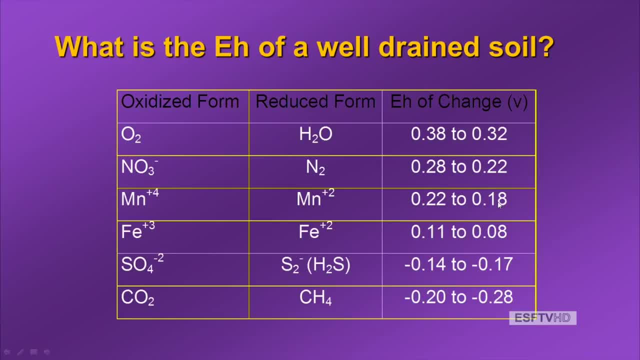 And eventually all that manganese is reduced And iron is next in line, Fe plus 3.. So you remember manganese this is- you can visually see this by those myrus tubes- And iron plus 3, going to iron plus 2, we visually saw that by these iris tubes. 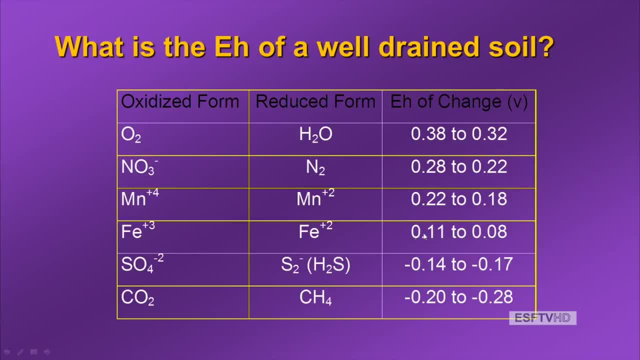 And the electron. the EH for that value is 0.11 to 0.08.. Now, eventually you can go through all the iron, OK, If these anaerobic reactions keep going, there's no more oxygen in the system. 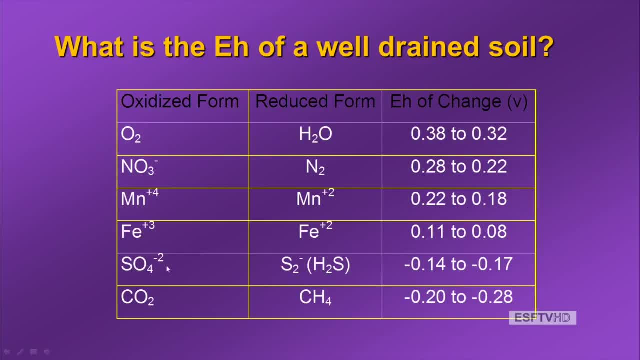 And then we end up with sulfate. So sulfate's next in line in terms of electronegativity to receive electrons, And sulfate- SO4 minus 2, is reduced to S2, the gas, And S2 combines with hydrogen sulfide. 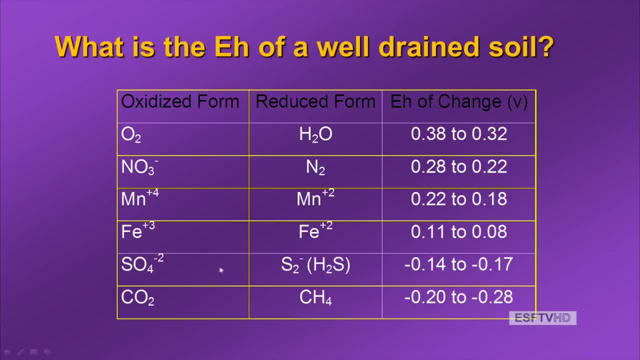 So you get the sulfide, And you know when that happens. that begins to stink, It smells like rotten eggs And the EH value for that is yet lower: minus 0.14 to minus 0.17.. OK, And you can eventually go through all the sulfate and get down to carbon dioxide, CO2.. 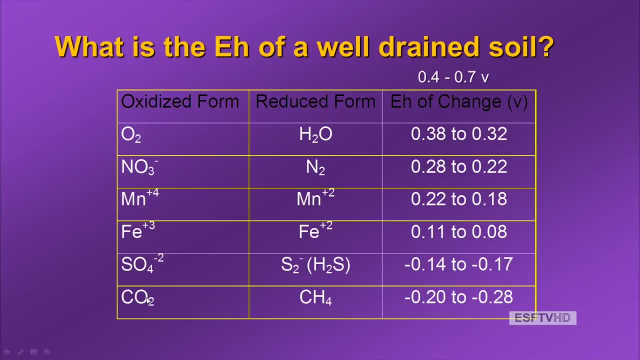 Now we're at a very low EH. Everything's been dissipated And CO2 is now reduced to methane. And you know methane- those little gas bubbles that bubble up in some of these swamps. You're looking at the process of anaerobic respiration, generating electrons. 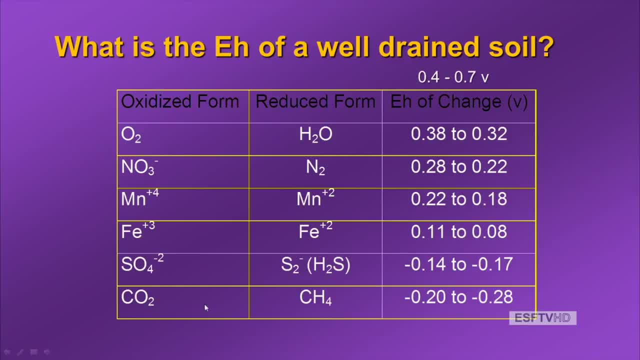 Those electrons being accepted by carbon dioxide and converting that to methane. And that's yet lower, minus 0.2 to minus 0.28 volts. So we can use these numbers to estimate the aeration status of soils. And so, if you ask, what is the question? 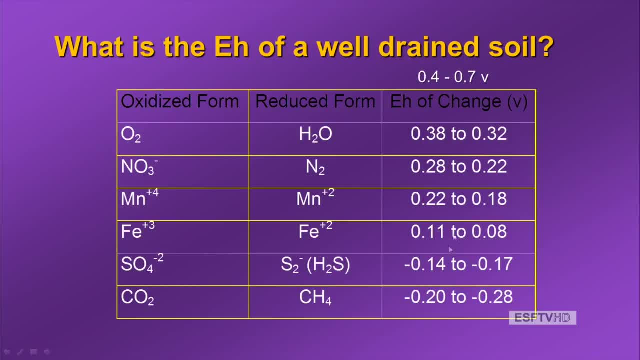 I'm sorry. You ask what is the value of EH. that is typical of a well-drained soil. We say it would have to go above that point where we have plenty of oxygen to be reduced to water, And so the EH of a well-drained soil is somewhere between 0.4 and 0.7 volts. 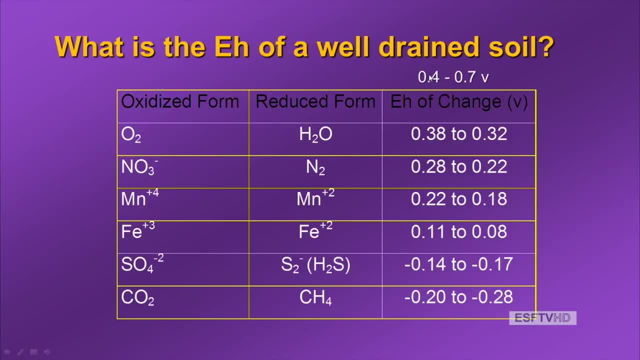 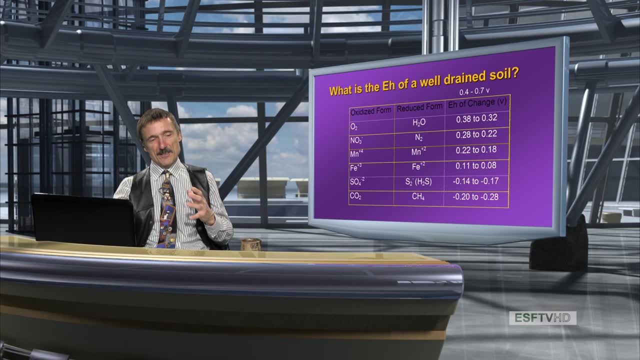 So this should make a lot of sense. I mean, this series should make a lot of sense. right, We start out with oxygen. We're in a well-aerated soil. We run out of oxygen. Nitrate is reduced. We run out of nitrate. 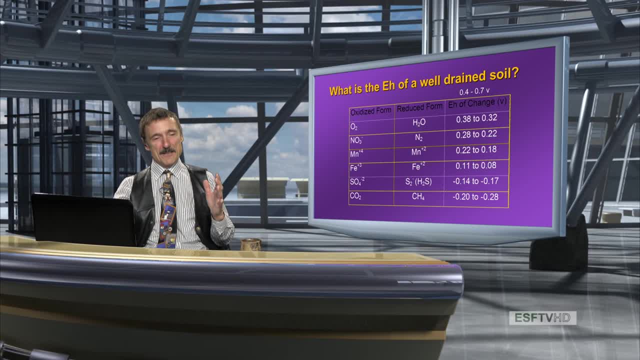 Manganese is reduced and so forth, until we finally get down to CO2 and reduce that. And so that's why in some of these anaerobic wetlands you'll see bubbles of methane coming up. You'll smell this hydrogen sulfide smell. 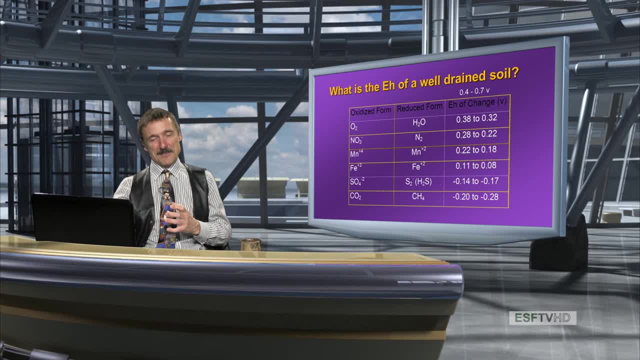 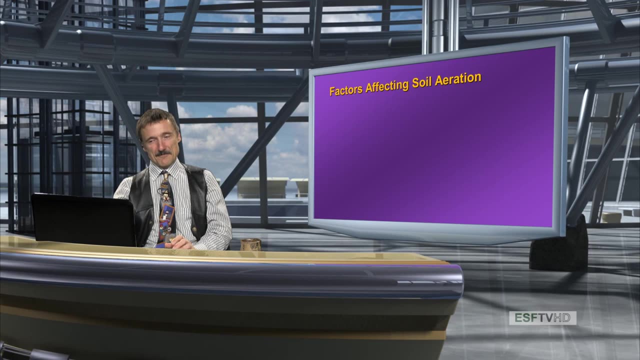 You'll see all this reduced iron, And this is why it happens. It's a successive transfer of electrons down to molecules that are successively more and more reduced in a very anaerobic system. Now we've got numbers, We've quantified it. 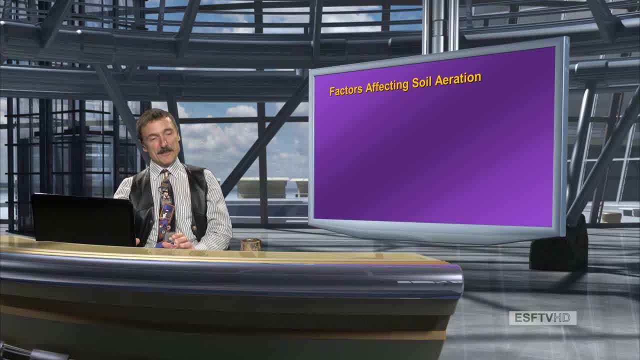 We have five ways to quantify it. And now let's think about the factors that affect soil aeration. Let's think about this in terms of the soil, So we'll move on to this idea, now that we can quantify it. So we think about what's the first thing. 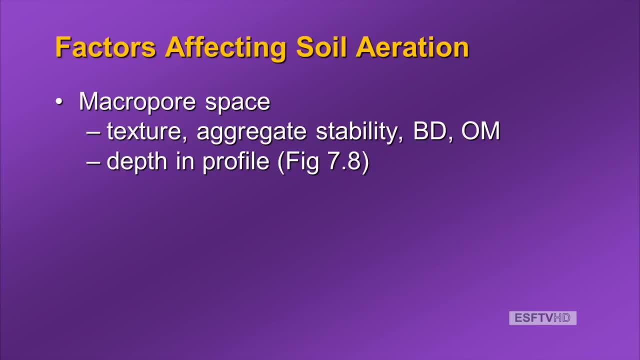 And we think back to our graph of well-aerated soil and macro porosity and air-filled pore space. And so we start to start. yeah, it's macro pore space. It's the amount of space that doesn't hold water against gravity. 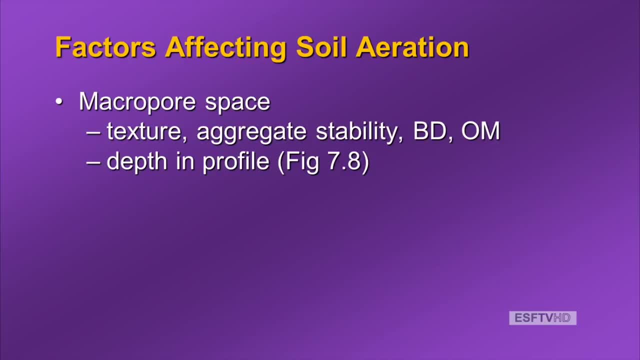 And we said in physical properties that was affected or impacted by soil texture, aggregate stability, bulk density and organic matter. All that kind of agrees and should line up really nicely with what we talked about in physical properties. So this add-on to physical properties is the next big connection with productivity. as we go barreling toward the end of the course, 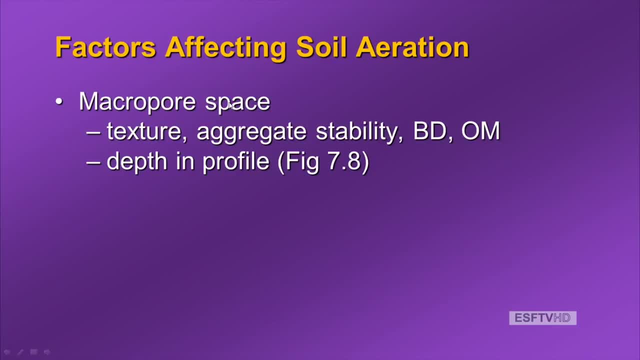 And so macro pore space, and we've already talked about those. in terms of soil physical properties. We've talked about texture, sandy soils. We've talked about aggregate stability. We've talked about those nice stable, water-stable aggregates and granules. 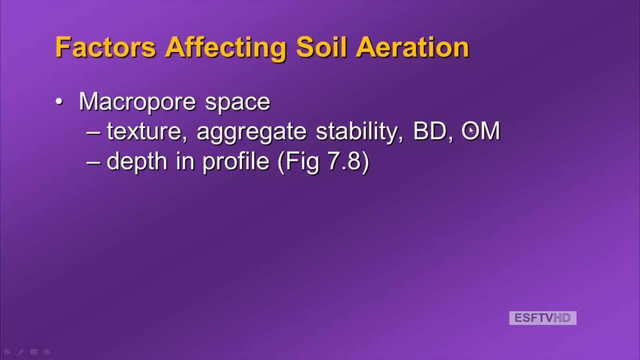 We've talked about bulk density, lower bulk densities, And we've talked about organic matter, Which has low particle density and which contributes to structure. So those are the physical factors that contribute to macro pore space And that's governing aeration. Again, macro pore space, more macro pore space, better aeration. 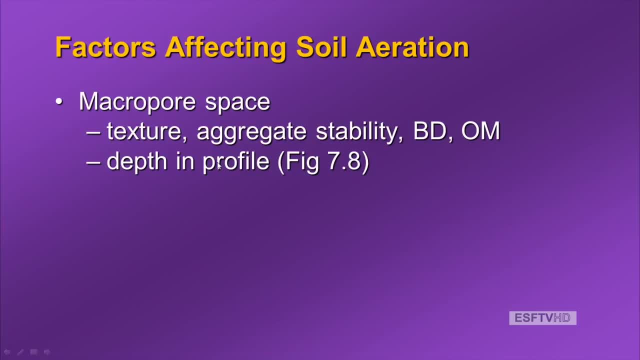 And the other part of that is depth in the profile. So as we go deeper and deeper in the profile, the bulk density increases, The pore size distribution changes, We lose those macro pores and those large mega pores And the aeration becomes larger. 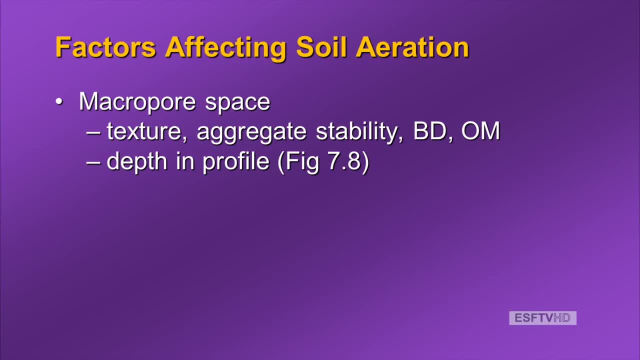 It becomes less good, let's say, Or it becomes poor depending on it, can even become poor, depending on these factors. And so that's the physical part of that. The biological part of this is the rate of biochemical reactions. So what's going on? 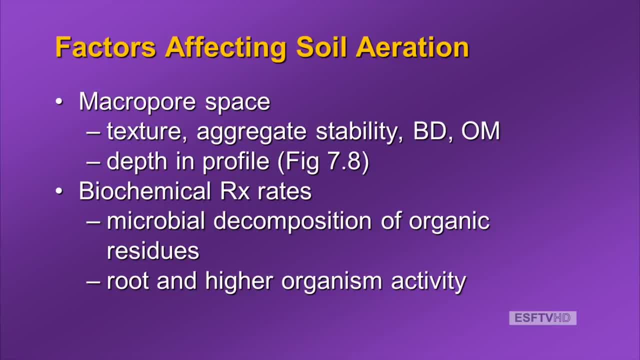 What's generating all this respiration? And largely it's microbial activity. Decomposition of organic matter, That's using up all this sugars, converting sugars to CO2.. And driving systems, Microbial decomposition, fungi, all these guys. And then what else is going on? 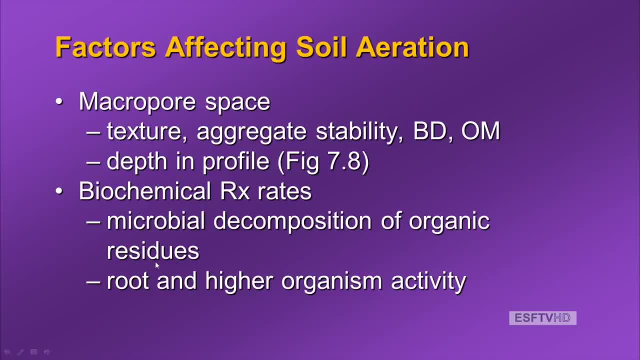 We have the root system And so roots and organisms, they're generating CO2.. So there's a lot of CO2 being generated. So as these rates increase the macro pore space, the rate of exchange has to rise to meet the occasion. 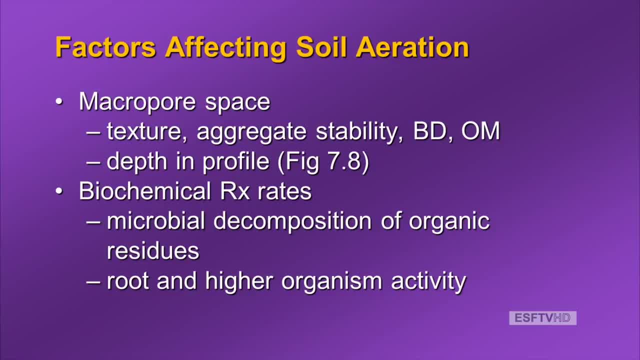 And when it doesn't, the soil becomes poorly aerated. So these two factors- macro pore space and biochemical reaction rates- are kind of driving some of this aeration. Now, if we look at this and we think about biochemical reaction rates, we've got to throw in season right. 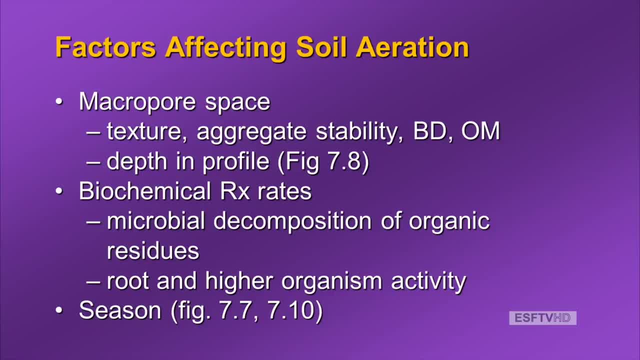 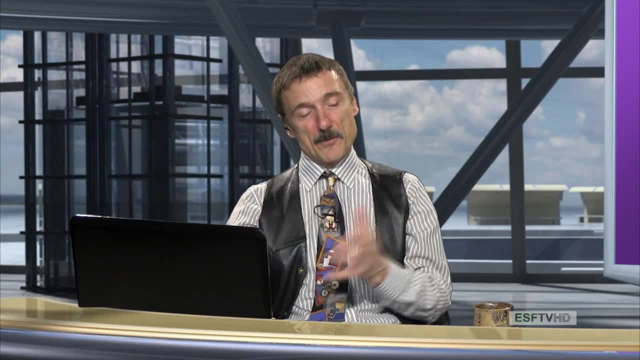 And for obvious reasons, We have a lot of biological activity in the growing season And we have a lot of biological activity And when you get away from the growing season, things slow down. So we can think about this in terms of a seasonal nature. 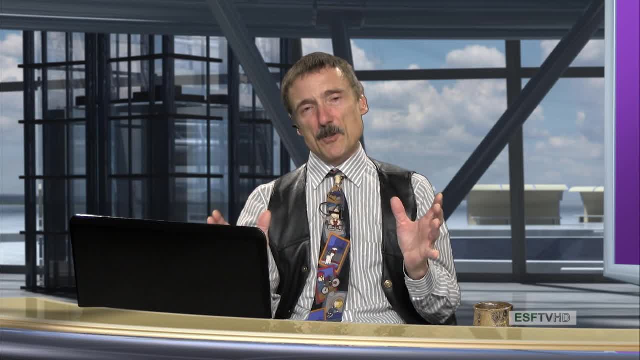 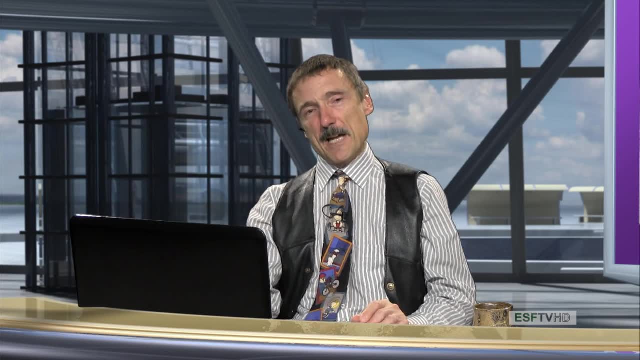 And we can explore that, We can think about this And to express this is carbon dioxide in a corn system. So let's look at what happens from this illustration of the text. Here's data from a corn field in Missouri, And it's seasonal. 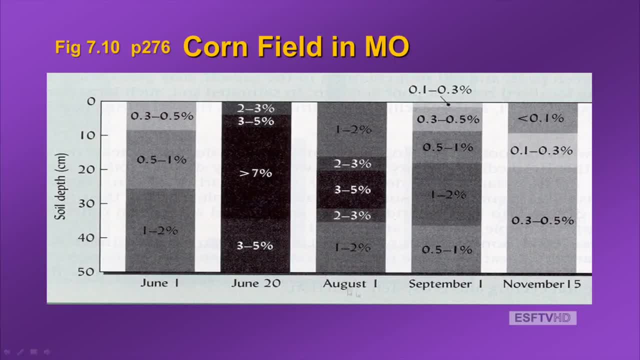 So we go from June to August, to September, November. So basically we go through the growing season into the fall season, when growth stops. And we're looking at this by depth. So on the axis, the y-axis, we have depth in centimeters. 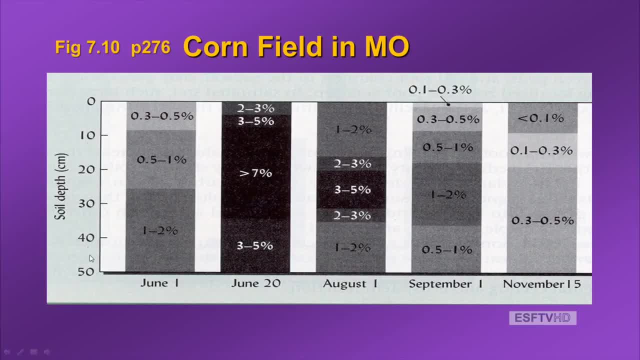 Up here at the top we're at the surface And we go down 10,, 20,, 30, down to 50 centimeters. That's half a meter. So if we look at what's happening in June and we see the pattern of CO2.. 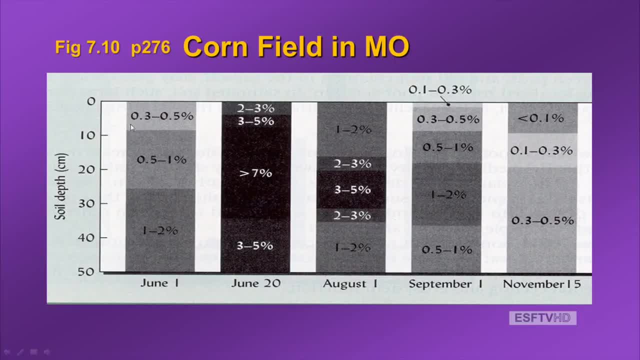 So this is CO2 concentration. This is a corn field. It's about 0.3 to 0.5% And it increases with depth, So this should make sense. We've got a lot of biological activity. As you increase with depth, the macropores dissipate. 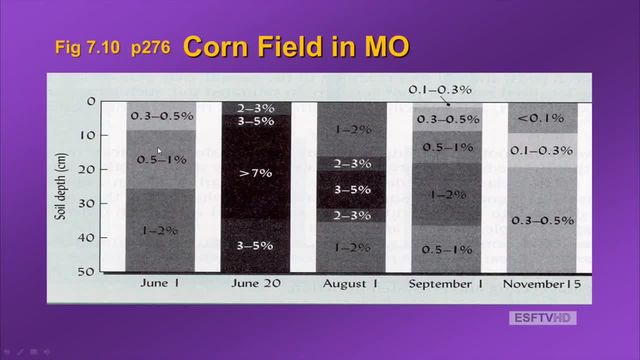 And things are just getting going And the concentrations are starting to get high, much higher with depth. Okay, So we go into the height of the growing season, the summer, when those corn roots are really putting out. Okay, Look at the pattern change. 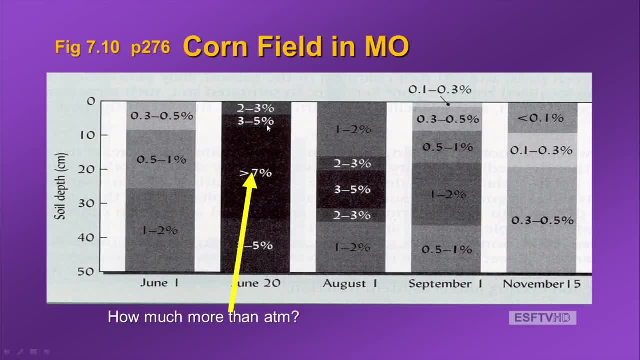 Okay, Now we're at the surface. We're 2% to 3%, 3% to 5% And we're increasing with depth tremendously. Right here in the middle of the root zone, we're greater than 7%. Okay, 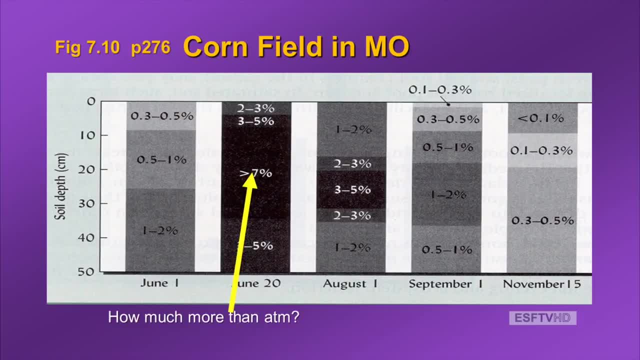 And it drops a little bit, So it's really highly concentrated there. Okay, 7%, How much more higher than atmosphere? So this is a question, a take-home question. The atmosphere concentration is what? 400 parts per million? 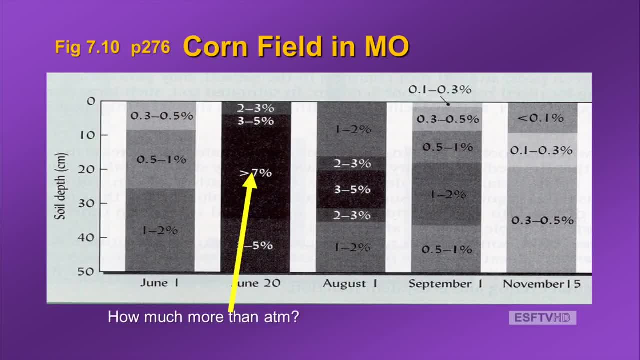 So I'm going to ask you, on an exam perhaps, to be able to tell me what is the? how much more is the concentration in the corn of 7% relative to this 400 part per million in the atmosphere? This is a pretty astounding number. 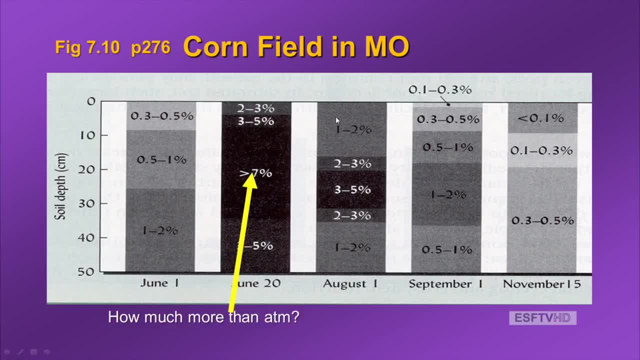 Let's go on with our season. We move into August, Okay, And notice what's happening. So August, the fruit. the plants are starting to fruit, All the corn is coming out, Root growth is dissipating. All that net primary productivity is being directed toward the above-ground parts. 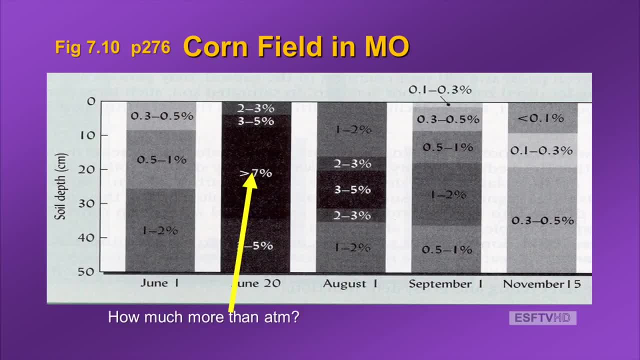 Okay, Root growth is slowing down. The CO2 is starting to dissipate, So we're seeing the reduced biological activity in terms of the roots And the numbers go down. Okay, And we're looking with depth, We still have a really high concentration. It's 1% to 2%, increasing with depth, 3% to 5%, But they're dissipating quite a bit And now we're getting a little lower in the very deep horizons. We get into September and leaf fall is going on. 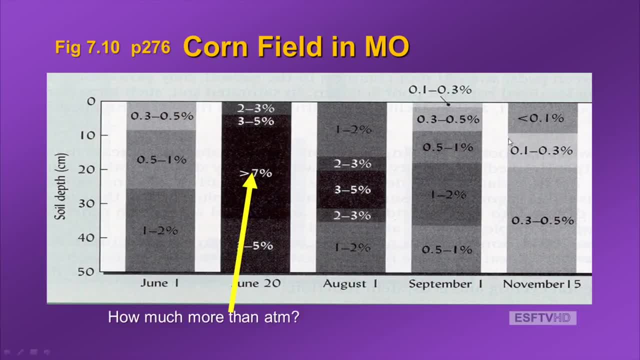 The plants are dissipating even further, The level of oxygen is improving, The level of carbon dioxide is improving And the numbers, the CO2 numbers, are going down because of diffusion And they are starting to really dissipate: 0.3% to 0.5%. 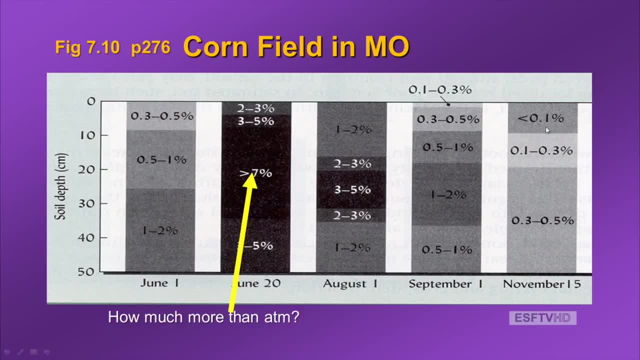 And as we move into the non-growing season, we're back down almost to where we were just before June. Okay, Less than a tenth of a percent: 0.1% to 0.3%. Okay, And 0.5%. 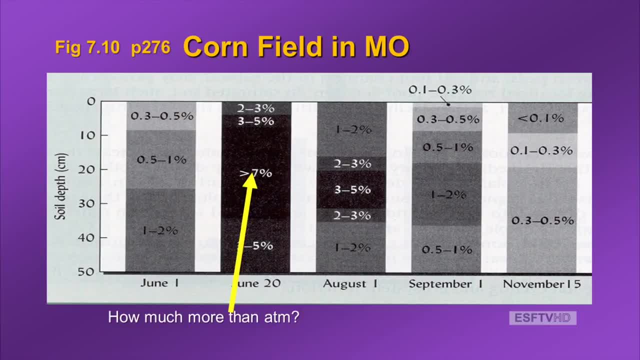 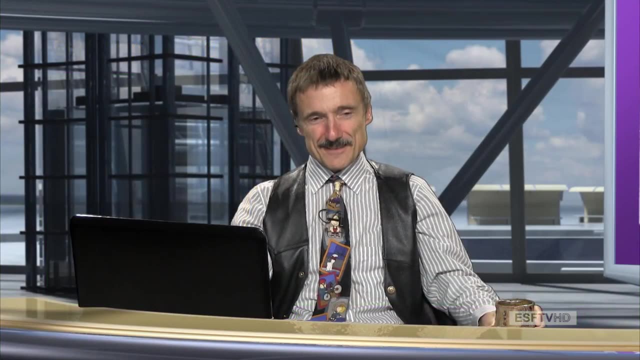 So this shows a seasonal pattern with depth. It shows increase due to biological activity. Okay, And a seasonal pattern with depth, And it's a very nice illustration of the interaction of depth and biological activity. So that's pretty astounding And so that's a corn system. 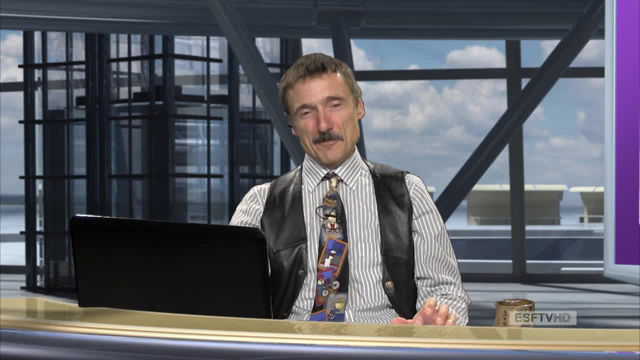 Let's think about a forest system. Okay, And a forest system again. we've got a corn system. Picture back to that slide I showed you in class, with very little in the way of macropores, And let's contrast that to a forest system where we have just a tremendous, ubiquitous number of macropores. 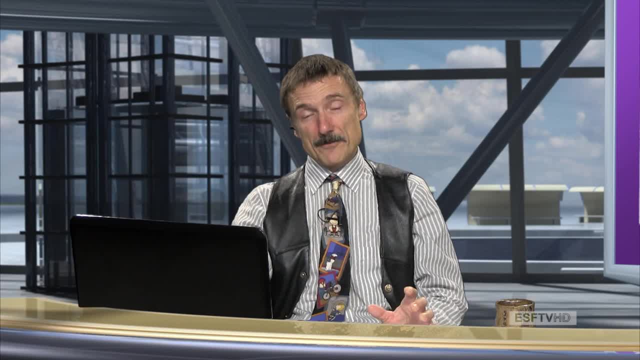 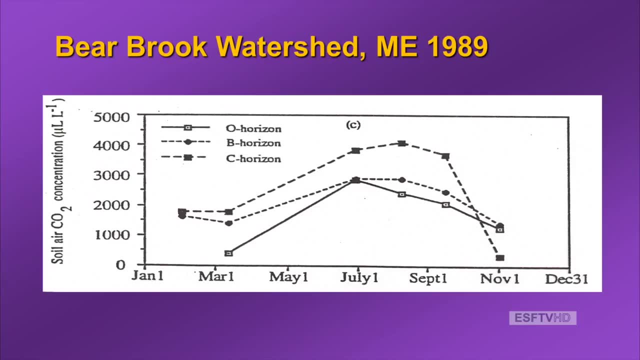 some 30% of the upper soil. Let's contrast this graph now with a soil system. Here we are from our Bear Brook watershed. This is up in Maine. some work we were doing up in Maine on some of these watershed studies And a colleague, Ivan Fernandez, provided this data. 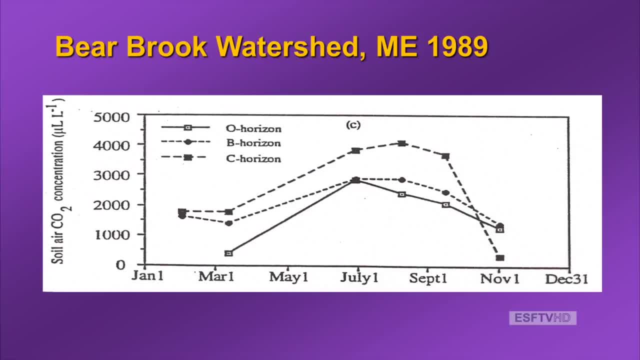 So this is soil air concentration: microliters per liter or parts per million on the left axis and it's seasonal. And now we're looking at by horizons, And so we have the O horizon by this square. Okay, And we go from March. 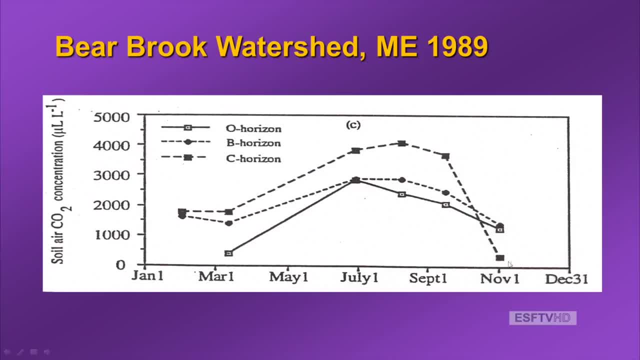 We basically go from winter through a whole season all the way to December And we look at the O horizon concentration of carbon. It's very low, Okay, Less than it's like 3,000, 2,000 parts per million in March. 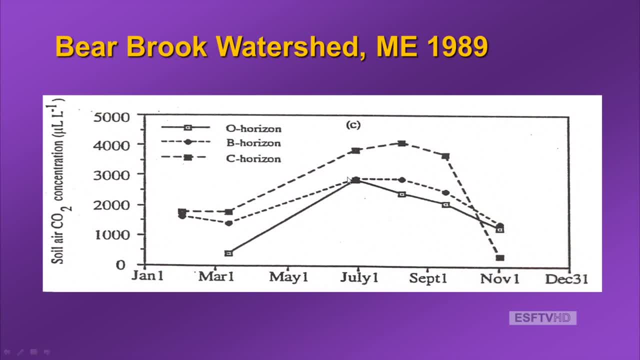 Biological activity heats up, Okay. And then we look at the B horizon- Sorry, 200.. It goes up to about 2,000 and drops down As the depth increases. the next is the B horizon. So we'll go to the B horizon. 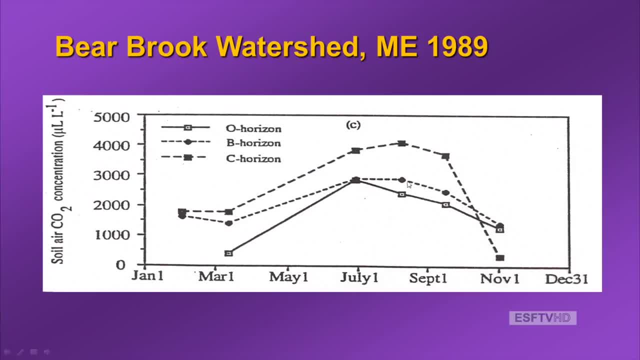 The concentrations increase. So that makes sense. Concentrations increase with depth, The macropore space decrease with depth, The rate of diffusion decreases, And so then we go down to the C horizon and the concentrations are higher yet, And in the peak of the growing season, just after root growth peaks at around July August. 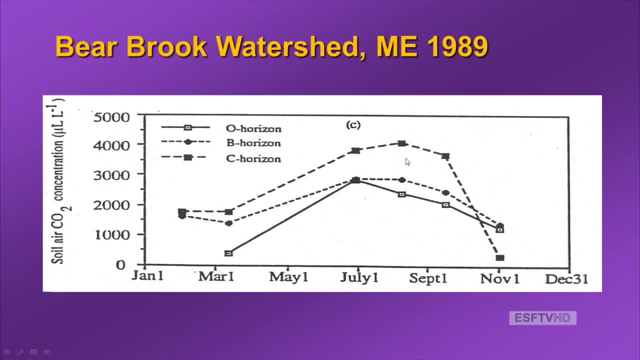 and then stops and then top growth ceases. here we have this peak, And so it's kind of neat to see the range of the height in the C horizon of about 4,000 parts per million. Okay, And contrast that to the corn example: 7%. 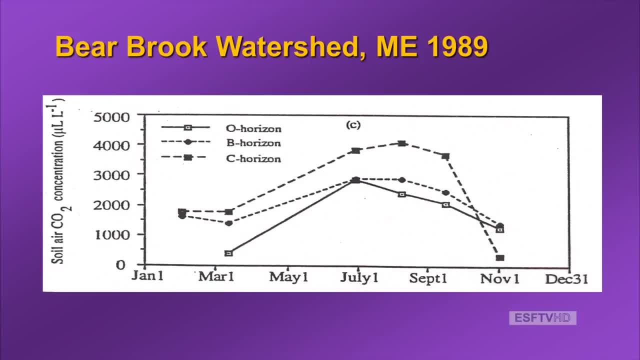 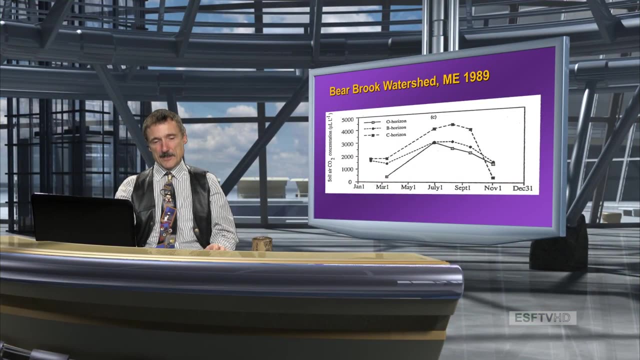 So a huge difference. Okay, That's a tremendous difference in concentration of CO2 due to ag systems and forest systems, And that's directly related to the amount of porosity. Both of these systems have tremendous productivity, But the ability, the capacity of the system to dissipate that CO2 is much, much greater in the forest system. Again, consider that about 30%, 20% of these huge macropores, large animal-filled burrows, and that's all absent in the ag system. So this is a really nice contrast of forest and ag, Both very productive: 400 bushels per acre of corn. 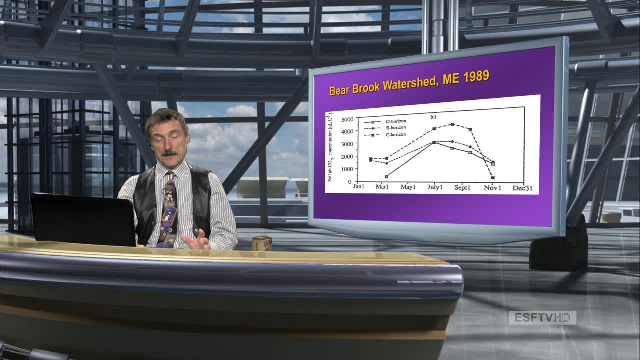 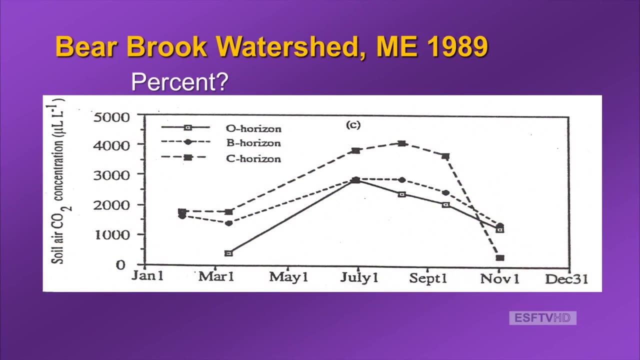 There are tons of biomass per acre or even per hectare of the forest system, But a very different picture in terms of aeration. So you should be able to convert parts per million to percent. So what is percent? Parts per hundred, Parts per million is 10 to the minus 6.. 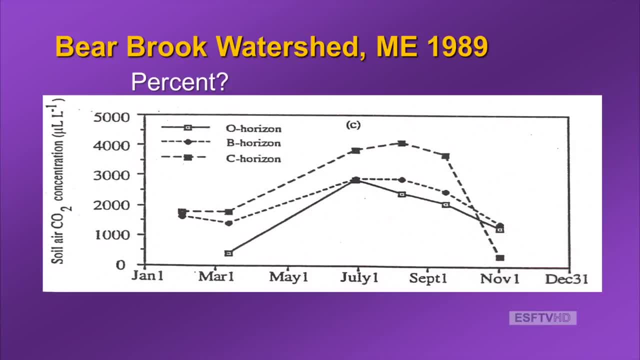 Parts per thousand, 10 to the minus 2. Order of magnitude: 4.. So I leave that to you, to be able to convert percent to parts per million. And then, how much more than atmospheric concentration. Okay, So remember the atmosphere. 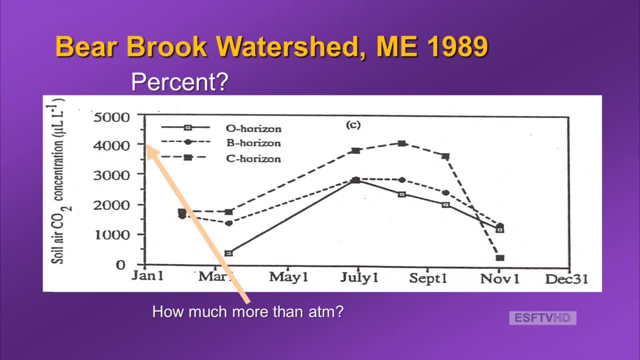 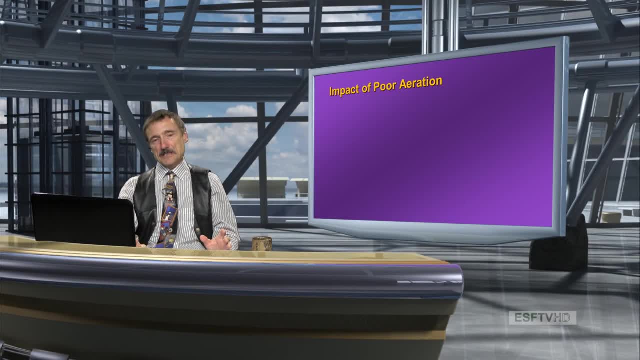 400 parts per million perhaps. So those are our numbers And let's think about the impacts. Aeration can be good, can be bad, It can be positive, it can be negative. So I won't put a value on this, but we'll kind of consider what that means for some of our systems. So let's think about productivity, Root growth, Root growth itself. poor aeration impedes that. So we start getting above that 10% CO2.. We start dropping below 10% oxygen. The soil, atmosphere And root growth is reduced. 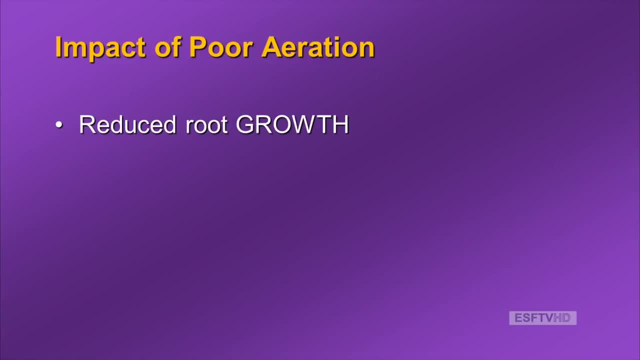 We drop below that oxygen diffusion rate of 0.2 centimeters, Oxygen is reduced, and so forth. 0.2 micrograms per centimeter squared per minute. So all those numbers drop below them and root growth is reduced. So it's not just the growth of the roots, 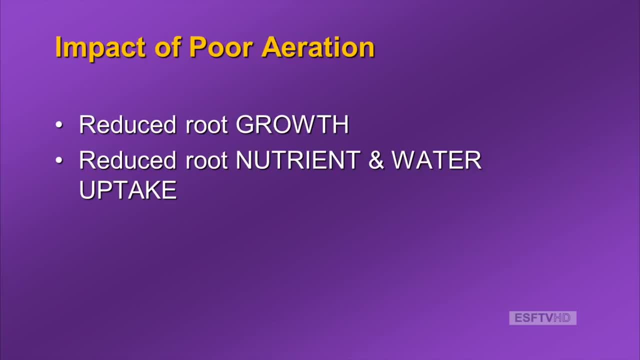 So remember the root is the uptake organ for the plant, for nutrients and water. So that is diminished. So poor aeration for most plants reduces root nutrient and water uptake. Again, there are plants that operate in anaerobic systems, but for the most part, for most of our aerobic plants, 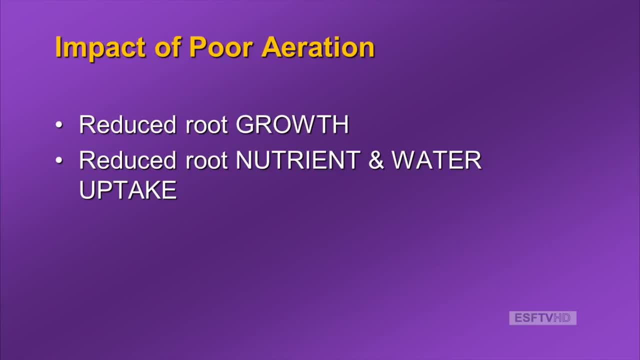 this is going to reduce nutrient water uptake. Microbial decomposition: Why does that matter? Well, the microbes are involved in releasing nutrients that are bound up in organic matter. So if we reduce the rate of decomposition, you reduce the rate of nutrient cycling. 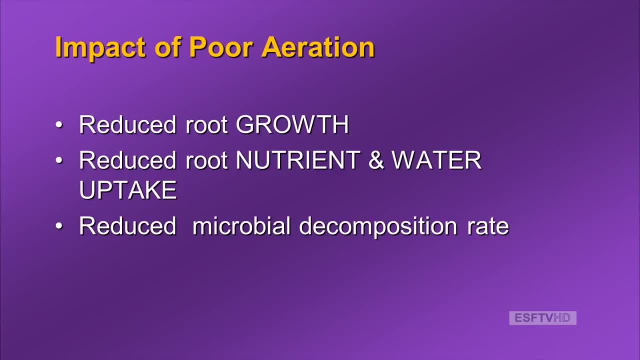 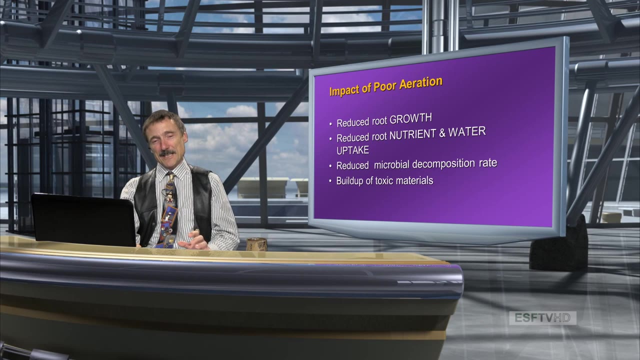 it reduces productivity. Toxic materials build up. What are some of the toxic materials? We talked about methane, We talked about hydrogen sulfide. Some of these are very toxic And, of course, if you've got a plant and you're starting to put out a lot of methane, 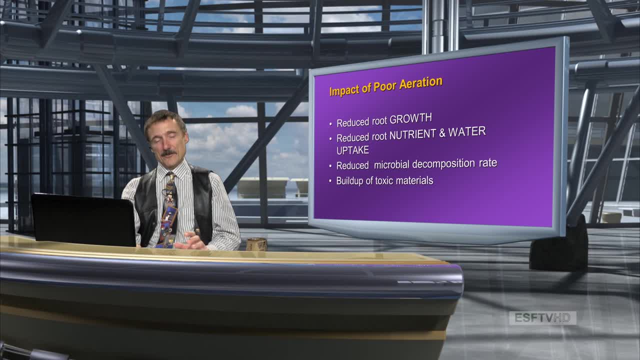 that's not doing anything for the roots. It's not contributing to respiration. Hydrogen sulfide: you're going to contribute to acidity. All these things that build up are not very good for plants, And CO2,, of course, is particularly not good. 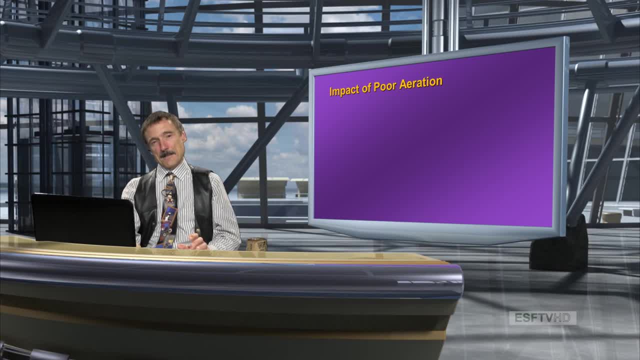 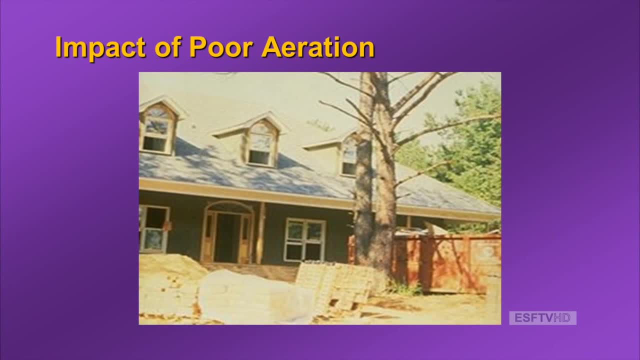 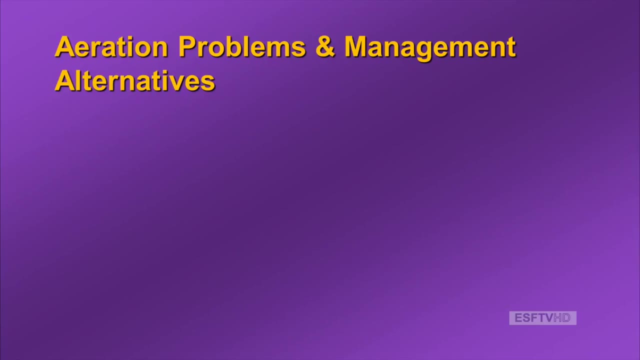 All right, Thank you. So some other impacts of poor aeration: Where do we go next? Here's an impact And this is a very positive impact. I would say it's kind of a negative impact with a positive outcome. if you're taking down trees. And so what do you do in a case like that? You're kind of up the proverbial creek without a paddle, But that requires a little bit of work. So when you get a contractor that doesn't pay attention to roots and compacts and poorly aerates, you have about a year or two before that is becoming history. 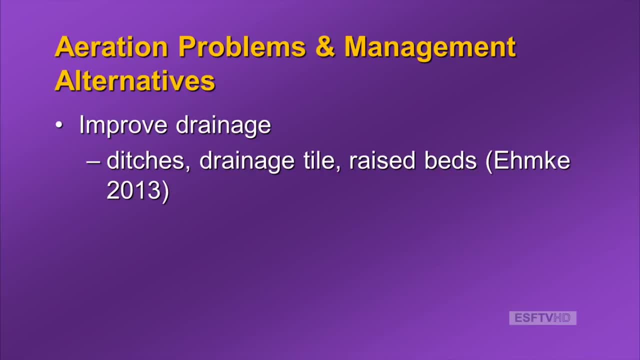 What can you do about it? So we like to live in systems where we have engineered solutions. So one solution to poor aeration is to improve the drainage, remove the water. How do we do this? Use drainage ditches, drainage tiles. 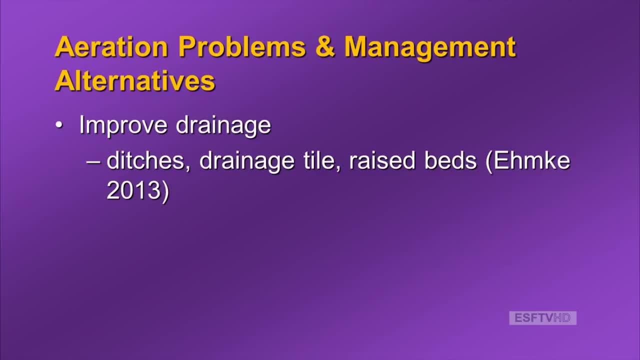 You can raise beds. Where did we see We were in a field lab. We went to a field lab where we saw quite an effort to improve the aeration. Remember where that was? It was the last field lab. It was at the DeSalvo Farms, where a system of ditches and tile drains in our organic soil. 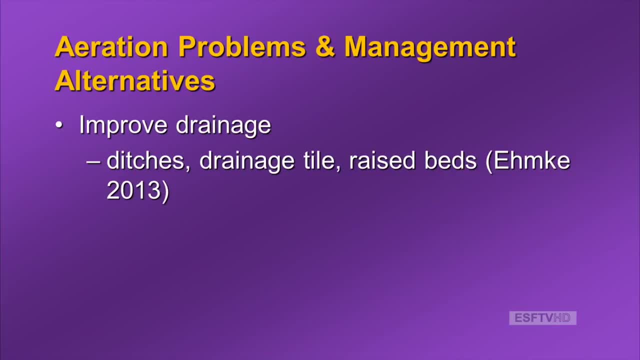 converted a wetland into an extremely productive agricultural land, And that was made possible by ditches and drainage tiles, reducing the water table or improving the aeration. You can also play with the hand that nature gave you and just manage for the appropriate species. 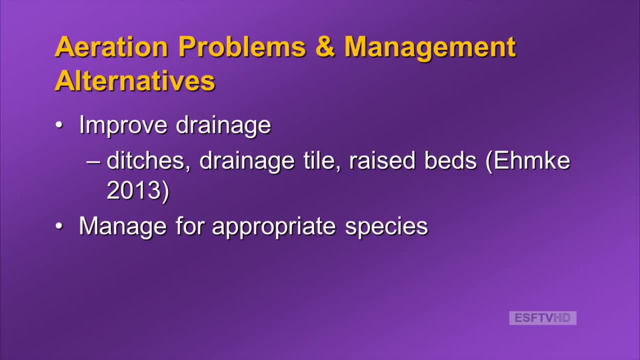 In a wetland situation. if you are managing a wetland, you're not going to favor aerobic trees, aerobic species, things like sugar maple and red pine. Maybe you're starting to look at things like red maple and some of the gum, some of the 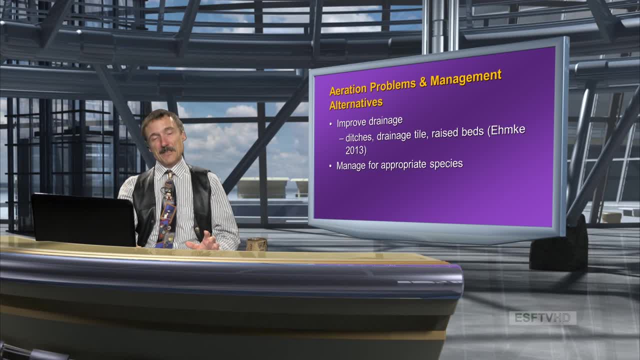 trees that can handle poor aeration. So if you have a little capital budget and a lot of land, you're not going to try and grow some of these species, like red pine, on a wetland, And so managing species becomes one of the big things. 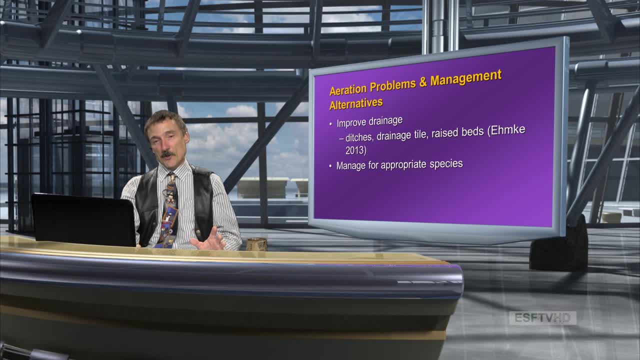 There are better ways or the most sane ways to do it. As you have more and more capital budget, as you move more and more toward an urban situation, you can afford to invest more money in reducing the water table Or, in the southeastern United States, the Lavallollie Pine Forest and the Coastal Plain. 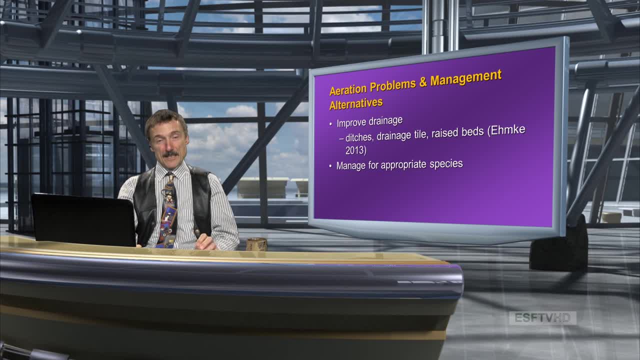 just to control the water table made the difference between a non-productive, non-commercial forest and a commercial forest, And only dropping the water table by about 50 centimeters made a tremendous difference in wood productivity, And there there's an economic return. 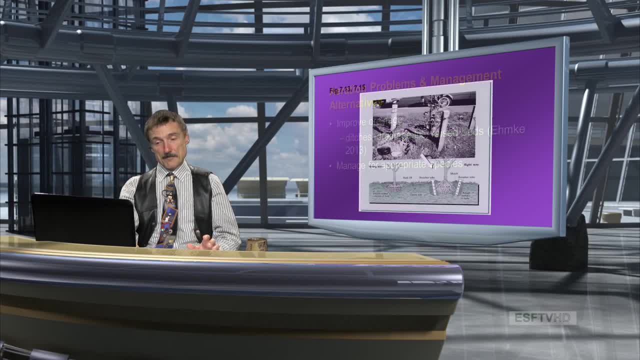 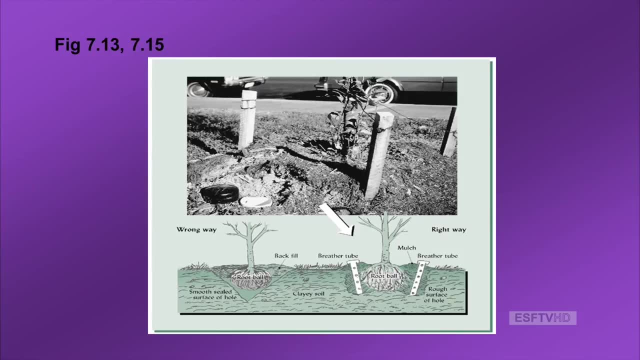 So that was a little bit of an engineering. Now here's what you can do for homeowners. You have lots of solutions and most of those have to do with controlling water table and digging out and providing drainage tiles. So one classic way to do this around trees and a lawn is these little aerator tubes, these breather tubes. 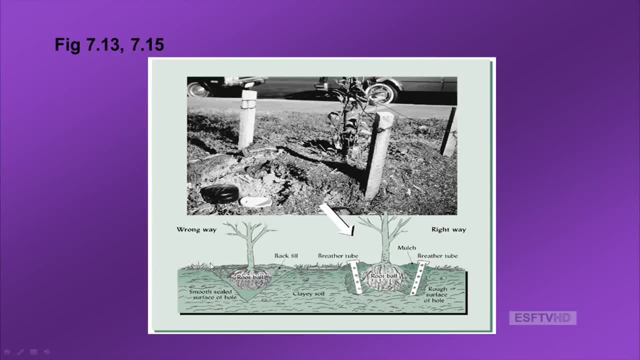 And note. this is a really nice the wrong way to do it. This is a nice illustration because this actually plants the soil. It plants the root ball in a ditch that fills with water. You have to have enough room for the roots to expand and grow and enough room for water to move through. 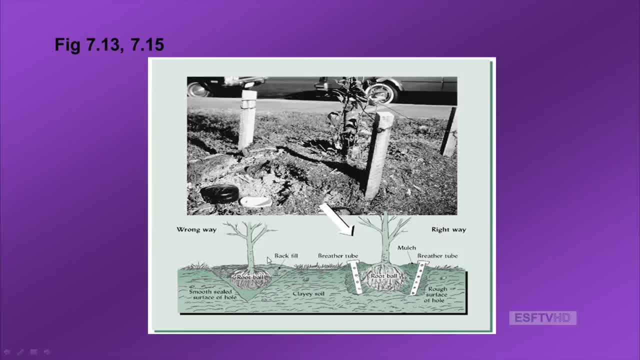 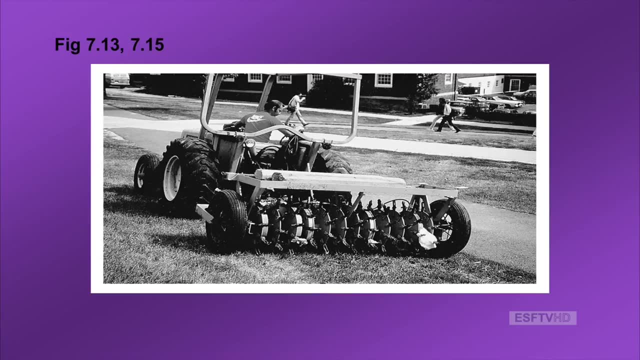 This is desirable. This is planting a death star, a death tree. So how do people aerate their lawns? Here's a little gadget that actually pulls out plugs. Okay, This is an aerator for a lawn, and if you just compress the soil you'd be changing the bulk density. 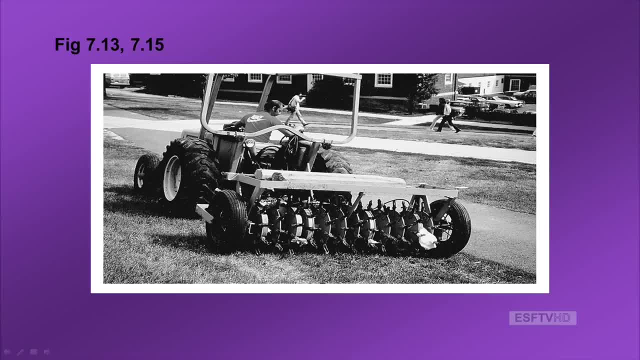 So this gadget actually removes little plugs and you drive this along and it pulls out a small plug and that creates a large gap, a macropore as it were, and deposits the soil, collects the soil, so that now you have a lower density and some artificial macropore space. 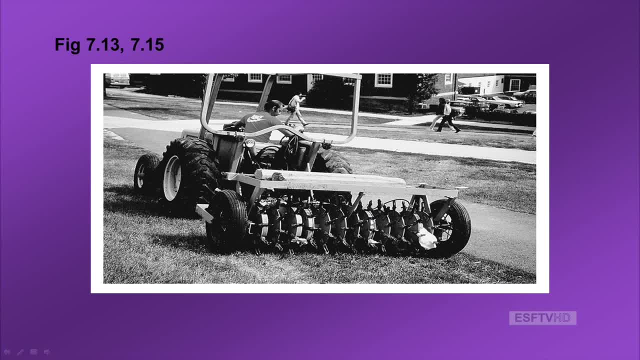 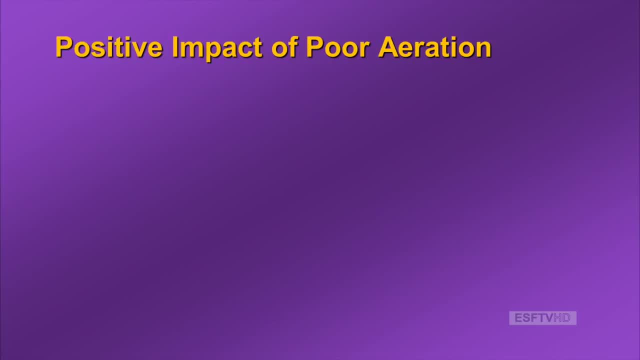 So this is an enhancement for turf, So it's not all bad, And so we've got to think there are positive impacts. There are places where poor aeration is desirable, And so we think about wetlands, And so wetlands are very important. 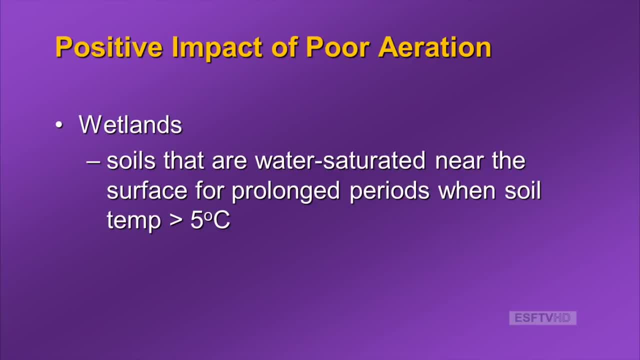 We've discussed those in our lab. We visited a wetland that was now a cropland and talked about the implications of making that a cropland. So we need a definition for a wetland. So if you look in the official core definition, this is it. 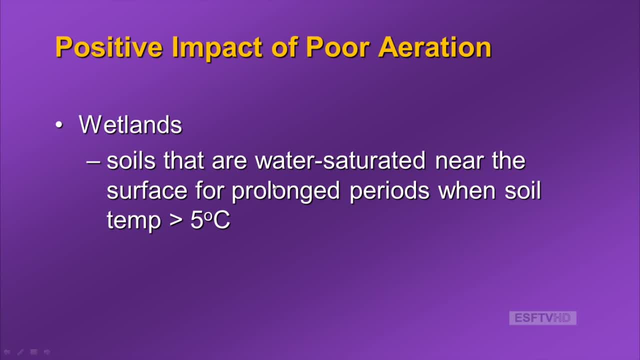 It's soils that are water saturated Near the surface for prolonged periods when the soil temperature is above 5 degrees C. It sounds like a lawyer definition, right? It's kind of nebulous: water saturated, okay, but near the surface. The question is how close to the surface Prolonged periods, What's a prolonged period? And another critical one that's pretty easy to see: temperature greater than 5 degrees C. So why 5 degrees C? Primarily because biological activity doesn't really matter. It doesn't really get started until you hit that temperature. So if you have a water-logged soil, no aeration and the soil is cool, it doesn't really matter. And it doesn't matter until biological activity starts up and respiration begins. 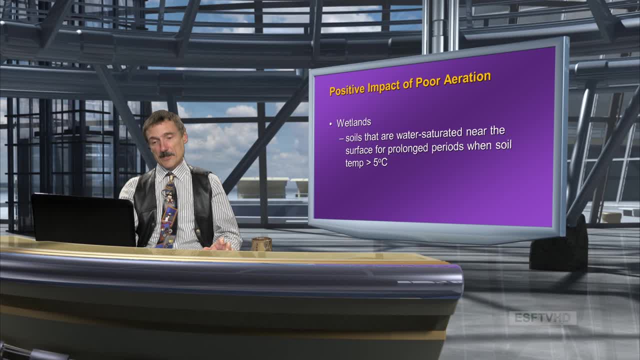 Hence this little piece here. temperature exceeding 5 degrees C. So that's the official definition, but we need more interpretation of it. It's just not enough for regulators, or to kind of hang your hat on. So we start to think: what is a wetland? 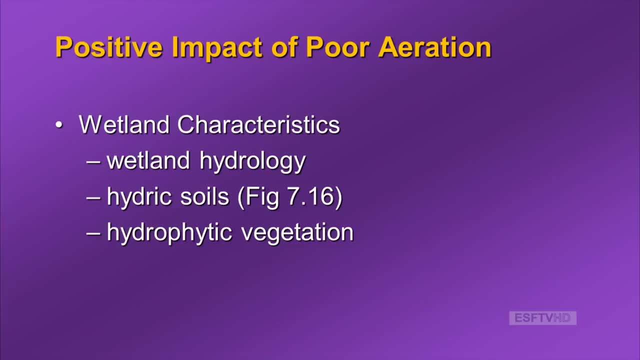 Wetland characteristics. there are three things used to define a wetland. These are regulatory criteria for wetland. One, that you have wetland hydrology. the water table is present. Two, that you have hydric soils. You say, well, I've got to define hydric soils. 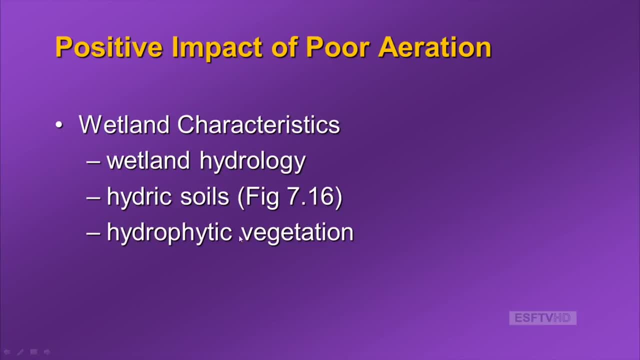 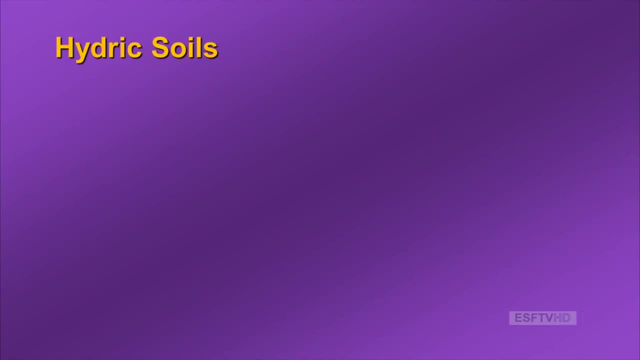 And three, hydrophytic vegetation. These are vegetation that will grow in anaerobic systems, So let's start with a hydric soil. Those are the three things, So you need two of three, two of the three, to identify a wetland. 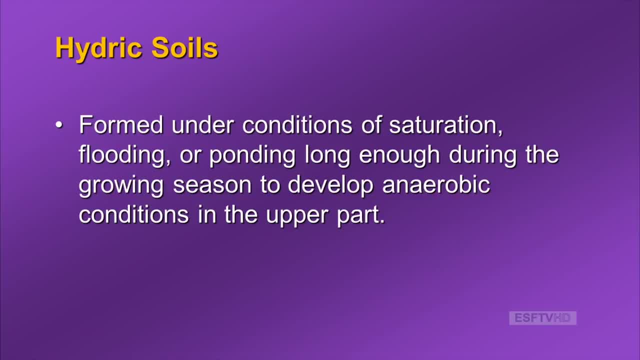 Hydric soil- another definition: Hydric soil are soils formed under conditions of saturation, flooding or ponding long enough during the growing season to develop anaerobic conditions in the upper part. Again, this is one of those. it sounds like it was written by a lawyer. 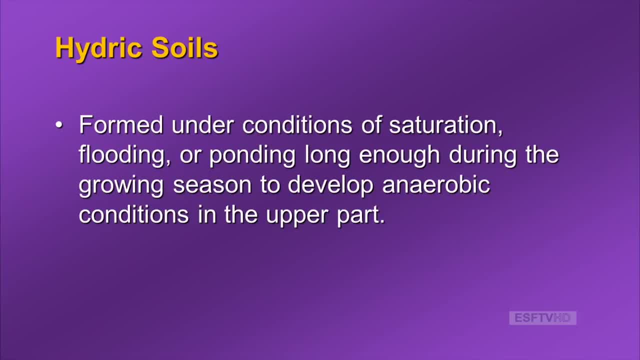 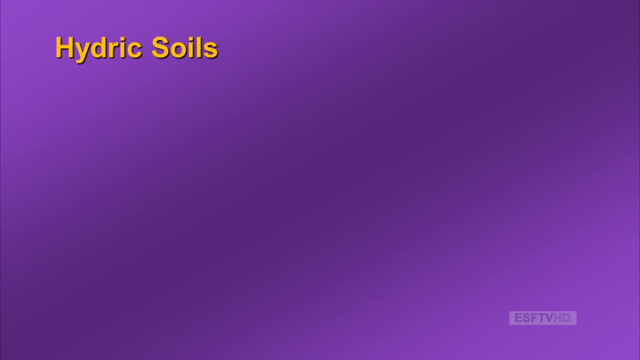 and so it's insufficient for managers. So we have to, we need more information. So the definition of a hydric soil, while it's informative, is not really useful for establishing criteria. So now we have to look at indicators. What are indicators of hydric soil? 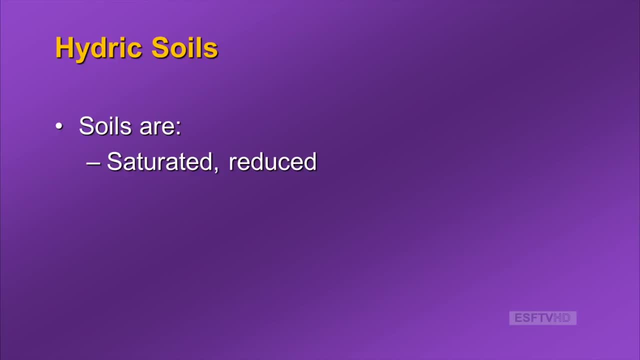 Soils that are saturated and reduced. That's fairly easy. You can tell a saturated soil, you can tell a reduced soil. But how We use hydric soil field indicators. So these are indicators that are based on soil morphology, And soil morphology is strongly impacted by reduction. 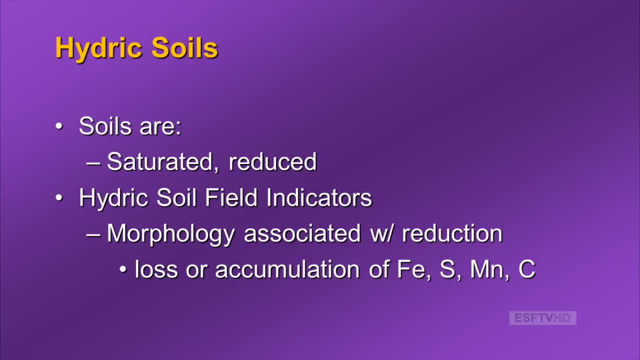 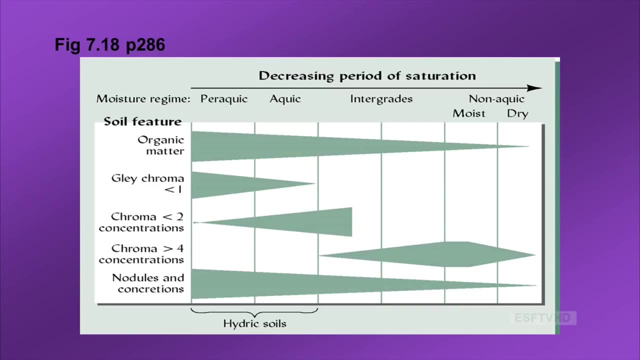 Soil morphology is strongly impacted and you can see it in terms of what accumulates Iron, sulfur, manganese and carbon. So let's focus on these as indicators of hydric soil. This illustrates it nicely. This is an illustration of color changing color. 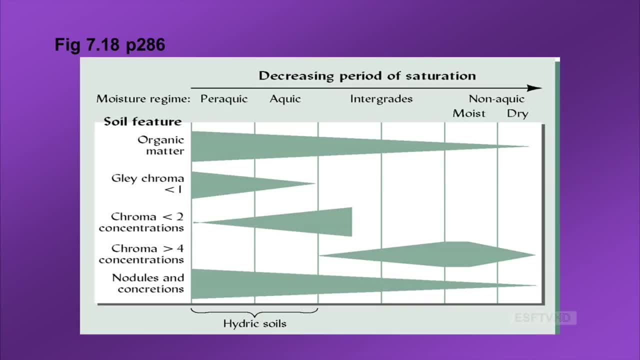 And organic matter buildup. So per aequic and aequic. per aequic is like a marsh Aequic is a wet regime, reducing regime, And then we get to non-aequic And note what happens. 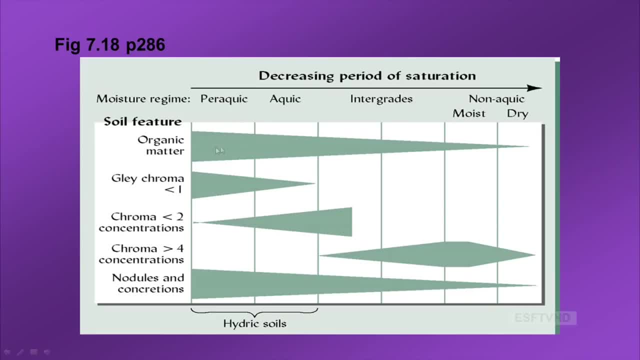 The organic matter buildup on these per aequic and aequic systems is very high. There's a lot of organic matter, a lot of carbon. The chroma is less than one. So remember why that is. Why is chroma less than one? 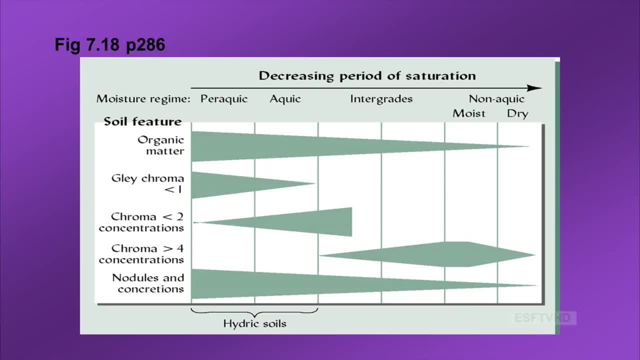 Remember iron, the story of iron and reduction. Reduced iron is glai or gray and a low chroma, And we talked about low chroma models. We also talked about chroma concentrations models. So this is a whole matrix: a glai chroma, less than one. 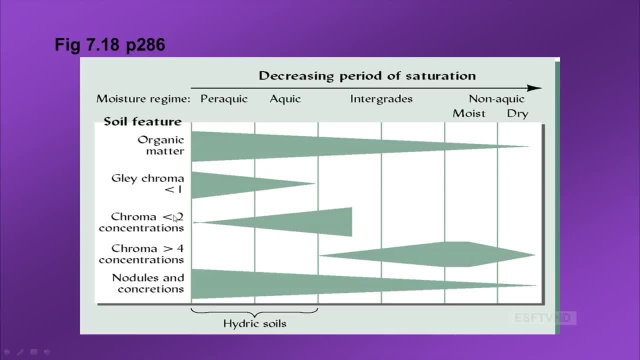 Concentrations, modeling chroma less than two. So look in the wetland piece. These are pretty highly concentrated glai chroma in these hydric soils. And we look at nodules and concretions. So a nodule. 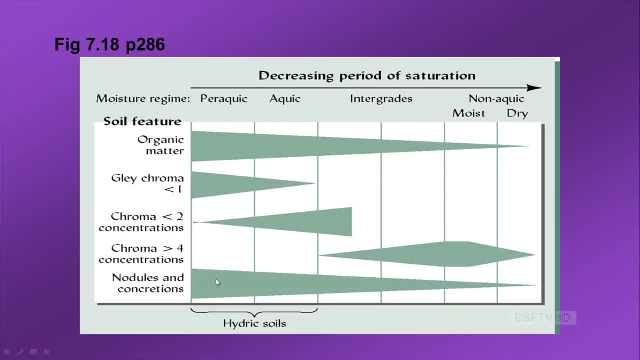 A nodule is a small, it's like a little BB And a concretion is like a layered BB, And these form in poorly drained soils. And so these are the characteristics. These are indicators of hydric soils, High organic matter, glai, chroma, some modeling, and nodules and concentrations. 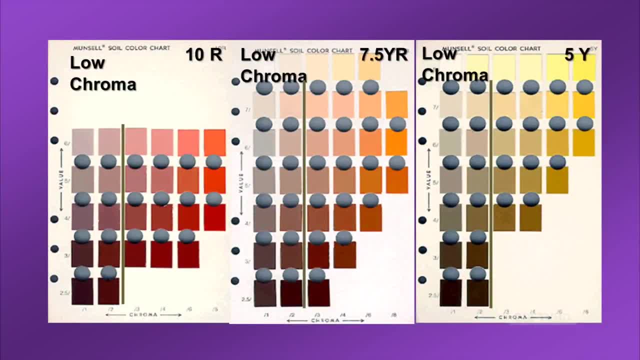 These are indicators. Remember low chroma. We go back to our Munsell color chart, Low chroma. over here on the left, One and two Low chroma, these left columns. And remember this is the U, 10R, 75YR, 5Y, the amount of yellow and red. 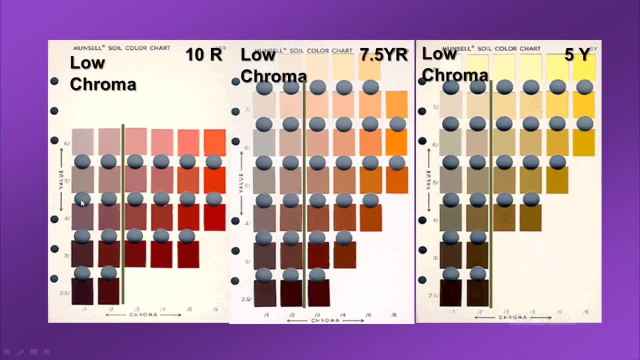 And for anything on the lower left, two columns is low chroma, these gray colors, And they have different expressions for different U's. So you go to the Munsell color chart and you can identify low chroma. Here's an illustration. 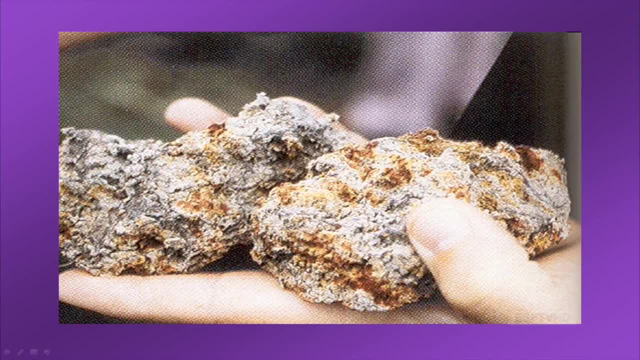 These are low chroma, This gray color, And that's too bad pixelated here, This gray. So this is low chroma. This is chroma one and chroma two. We have some modeling here. This is an indicator of a hydric soil. 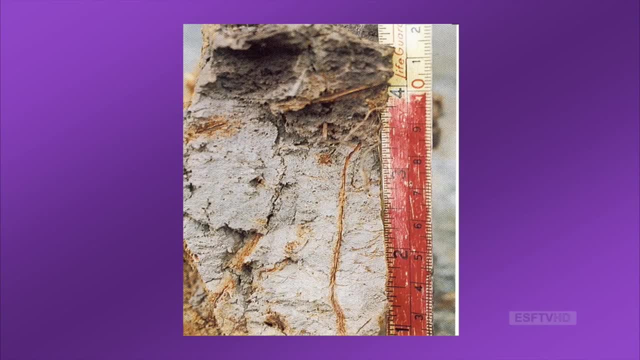 Should look familiar. Here's another indicator: oxidized root spheres. We have this glai matrix and this oxidized root sphere, So oxygen is transported to these plants that have erythema cells And that oxygen, That oxygen then goes to the outside. 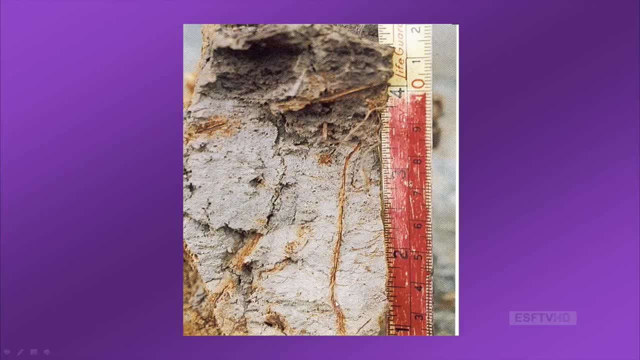 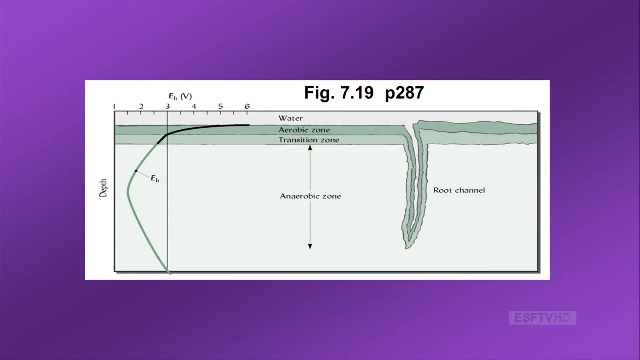 So just around that root, where the oxygen is present, you get the oxidation or the color of orange compared to this gray color. So let's take a look at what that last picture is on a graph. So here's water, There's a slight bit of aerobic zone. 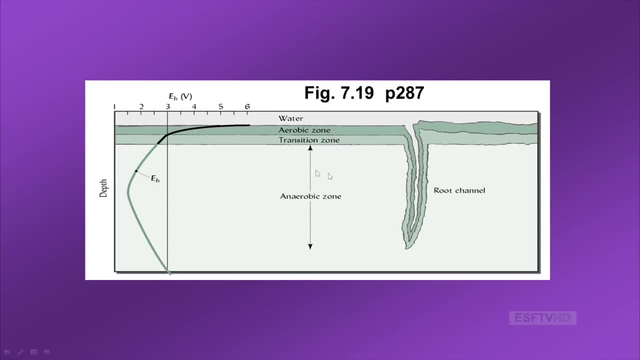 There's a transition zone, Then this anaerobic zone. There's all that material, all that oxygen dissipated, And here's what it looks like. The EH takes a big drop, Goes to small numbers. So we know that indicates a poorly aerated soil. 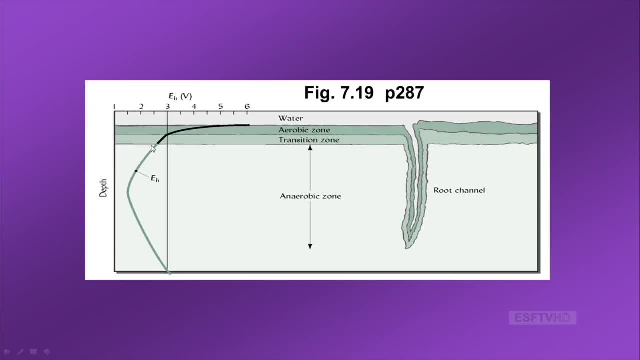 Smaller EH, And remember what's the reference. What's the EH of a well-drained soil, of a well-aerated soil? And we're looking at 0.4 and greater. So this kind of makes sense. It depletes with depth. 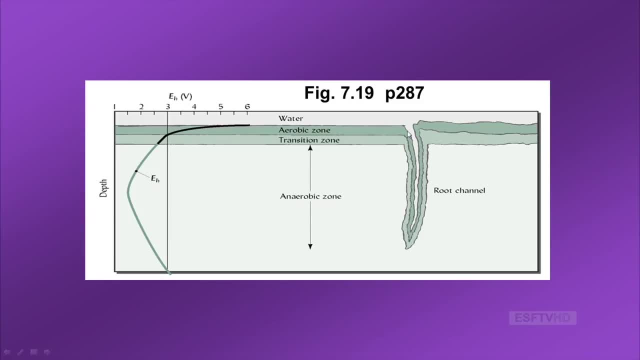 The anaerobic zone And we look at the root channel, And so you get this aerobic zone, This aerobic zone right around the root channel, because oxygen is pumped out to the roots through these arrhinchema cells. Then you get this oxidized iron. 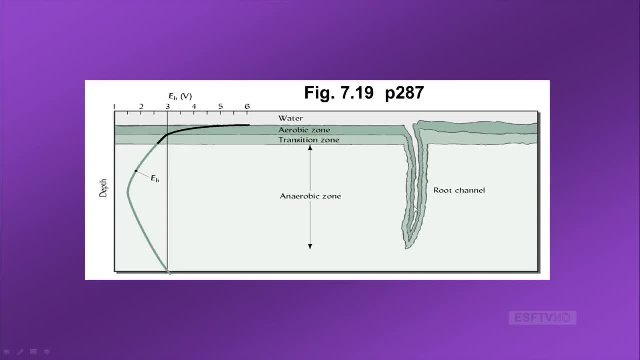 And then you have the gray around it. So this is a visual graph. Kind of matches up with the picture on a previous slide. Here's where the red would be, Here's where the gray would be And it's superimposed on that the EH oxidation reduction potential. 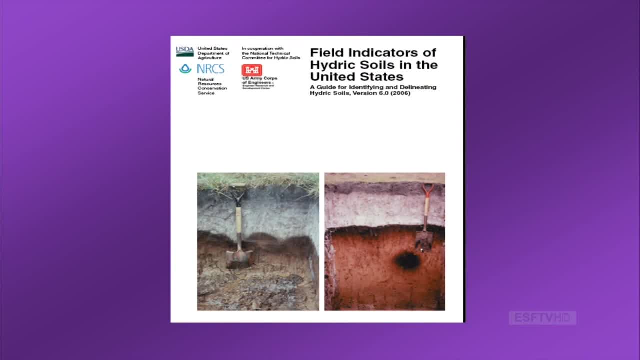 That's kind of cool. So where is all this information contained? So there are many hydric indicators and changes in different regions of the country, So we can give you this field indicators of hydric soils in the United States. So I have that linked on the website. 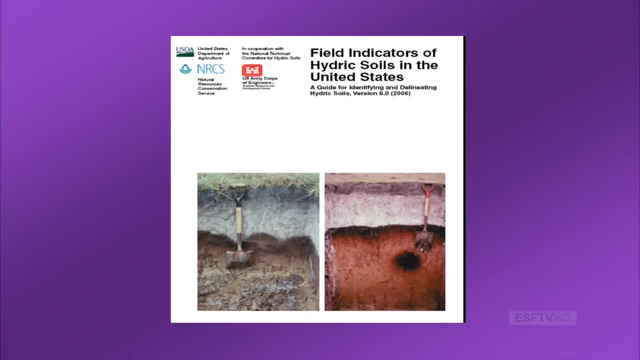 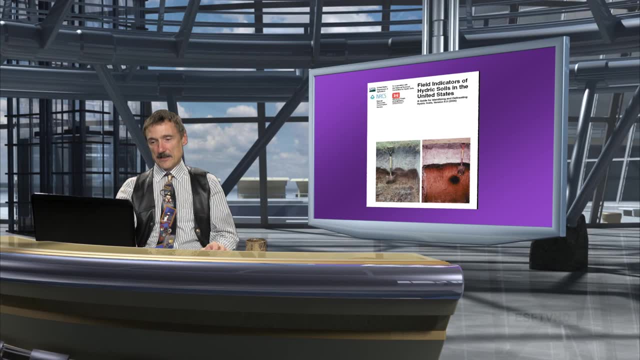 So if you're interested in, you can check that out on the website and get it. It's a free download. You can also order it from NRCS. It's a pretty useful publication And this is now what's used to identify hydric soils. 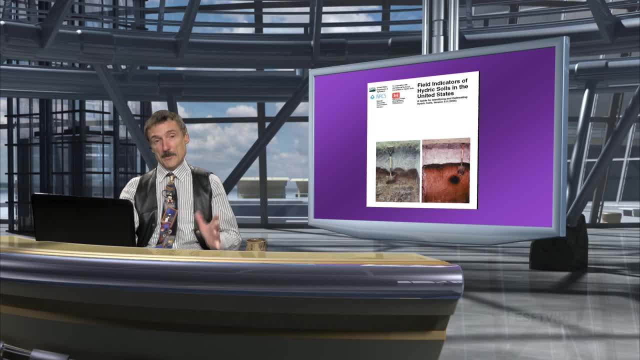 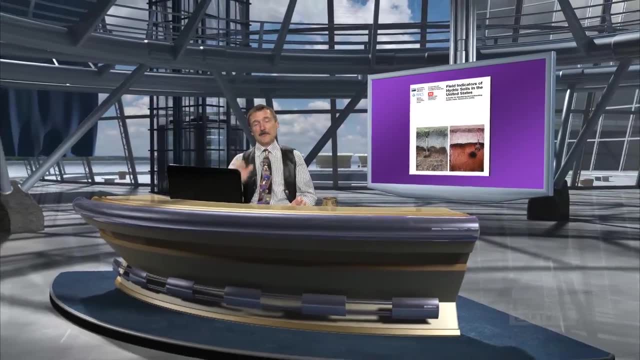 So if you get involved in delineation of soils and hydric soils and wetlands- and some of you might do this for a living- When you get done with your degree doing these wetland delineations, you'll become very familiar with this book. 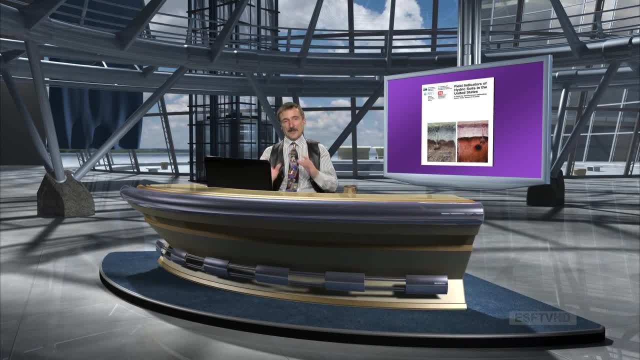 And for various parts of the country and various types of the soils. there are a number of indicators And they're all collected here And they're continually being tested and updated. Pretty cool, Free your government dollars at work So you might be a hydric soil if you have a depleted matrix. 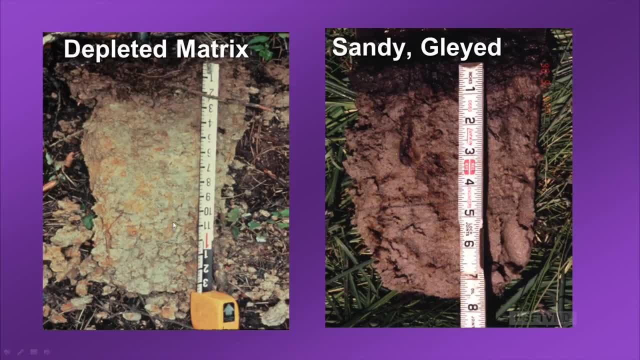 Here's a depleted matrix. It's depleted of iron and it's gray. This is called depleted matrix and it's a morphological indicator of color. Here is a sandy soil. It's glade, And the same result: this low chroma matrix. 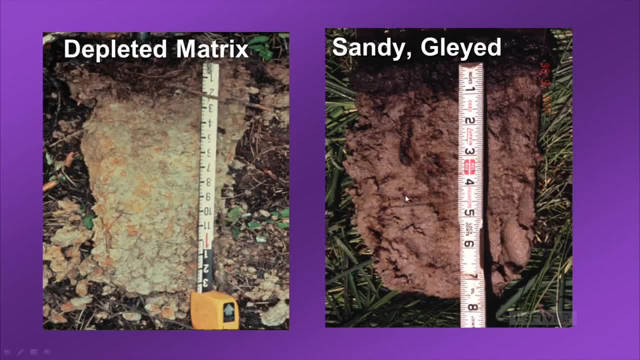 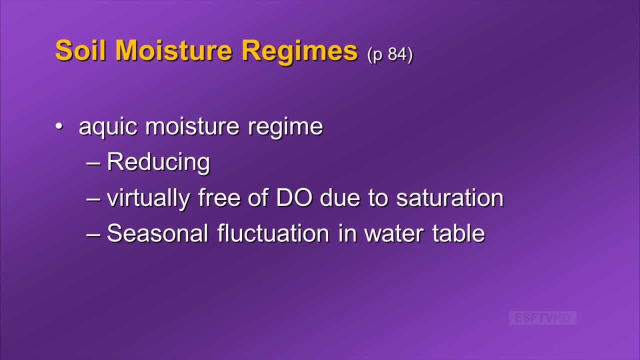 This is a hydric soil indicator, And so you see this condition and you check off: yes, this is a hydric soil And so kind of. we tie this together and think about the soil moisture regimes, Because I introduced the concept of aqueous and peraqueous. 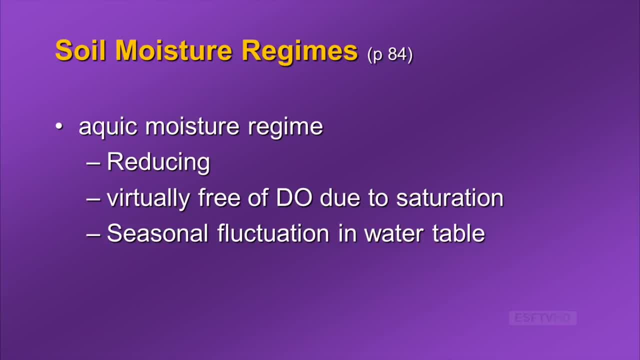 So let me back up and kind of define those regimes: Aqueous moisture regime, aqueous wet- This is a reducing regime And so this describes a condition of no dissolved oxygen. DO stands for dissolved oxygen, And why? Because of saturation. 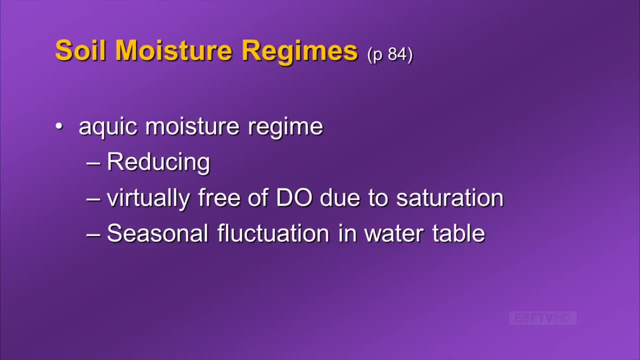 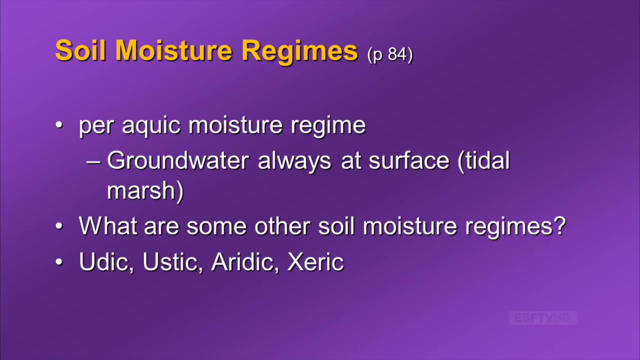 So saturation deprives the pores of air space, All the oxygen is taken up and there's none left. And now we have an aqueous moisture regime and a reducing condition- And this happens a lot- seasonally Peraqueous, So this is where groundwater is at the surface. 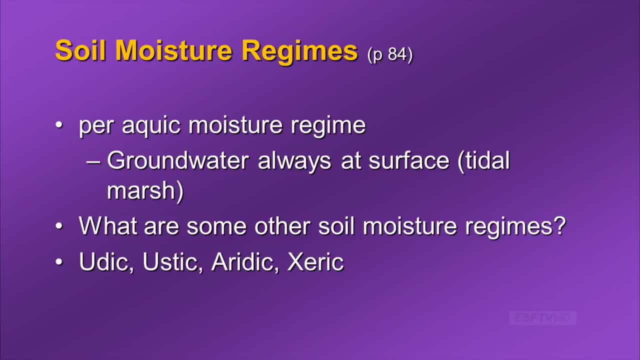 So instead of a seasonal situation, this is continuous. Groundwater is always at the surface And typically these are marsh situations. Do you know some other soil moisture regimes? If you think back to our exercise in soil water, our lab in soil water, you'll think back of several.